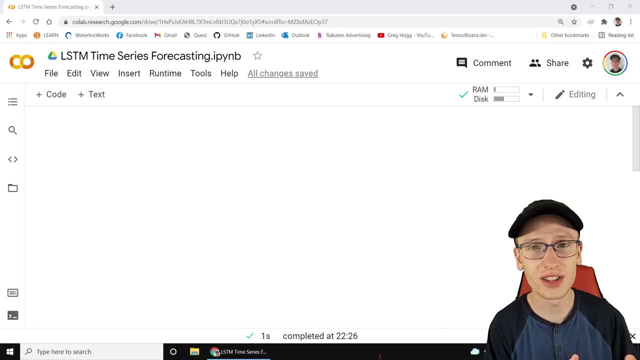 Hey everybody, how's it going? We have a very, very exciting video today on LSTM time series forecasting. So this is probably the most requested video on my entire channel since it started, and so, because of this, I really, really ask that you drop a like on this video, no matter who you are. 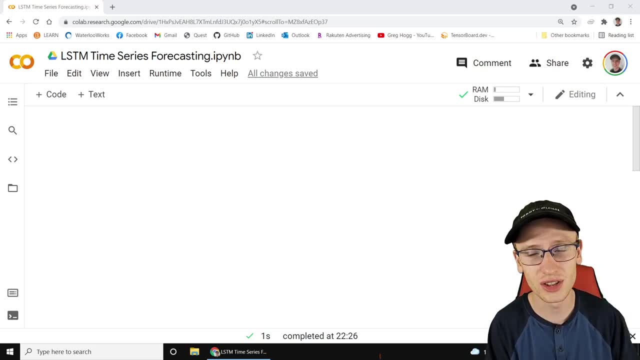 because I know it's a very important topic and it needs to be taken seriously and it also needs to be taken slow and nice and easy. So I'm here to explain that to you. Please go and drop a like on this video so it does nice and well and everyone can see it. So we're going to be forecasting the. 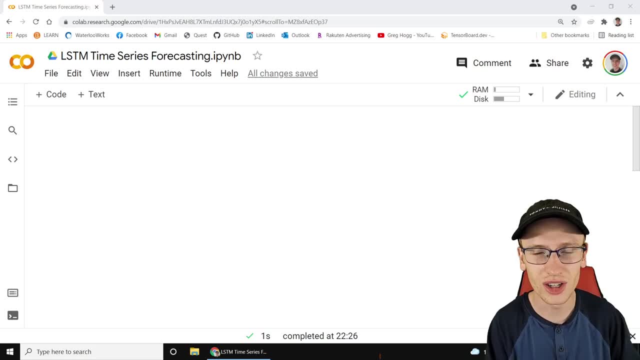 temperature actually Nothing like the stock market. We're not ready for that yet and if you really think you are, then go ahead and go do that. But today we're going to be taking it nice and slow and forecasting basically the temperature. So we're going to start out with our import. 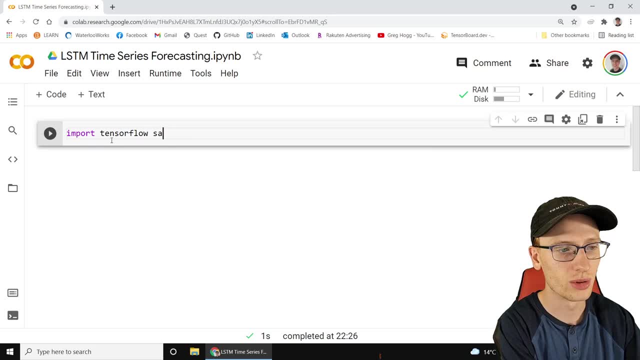 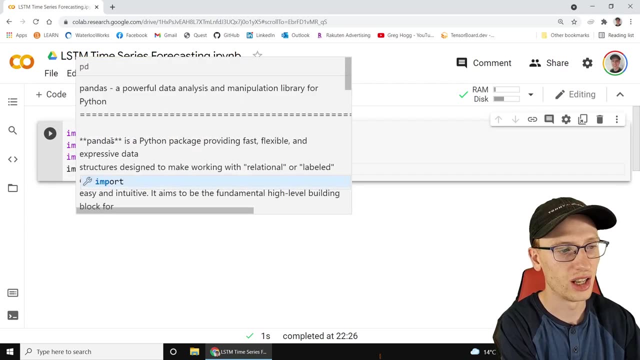 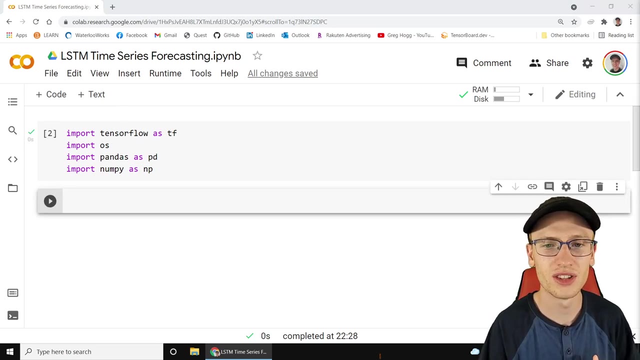 statements: as usual, We're going to be using TensorFlow and we'll import that as tf. We're going to import os. We'll get pandas as pd and numpy as np. Okay, that's pretty standard, And we're going to now just copy and paste this thing to get the data set. I don't really want. 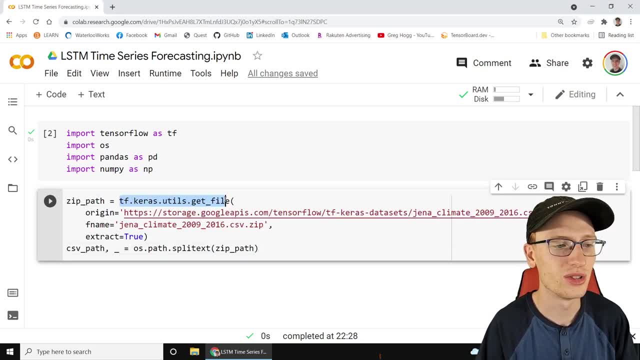 to bore you with showing you all the details here, but I'll explain it Basically. we're using the TensorFlow cures utils get file to get it from this data set. here You can see it's from TensorFlow data sets and it's going to be about the climate, which is, you know, going to include the temperature. 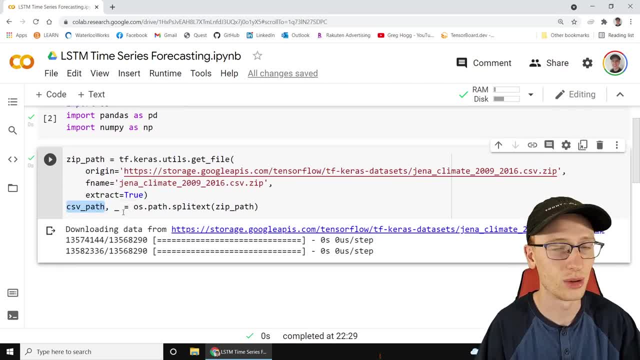 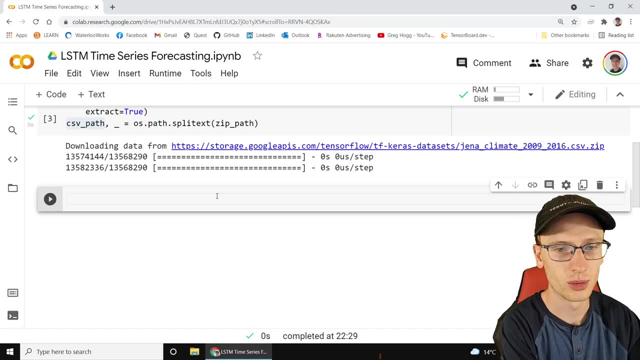 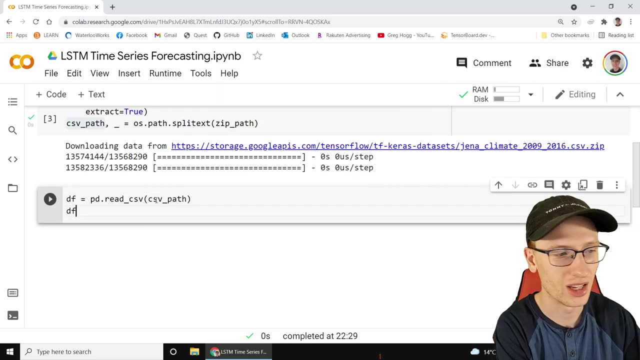 as well as many other things. So we'll run that and the most important thing is that we got this CSV path. So the CSV path. it's going to allow us to basically load this in as pandas. So we're going to call it as usual. df is equal to pdreadcsv with the CSV path and df is right there. Okay, so I'm. 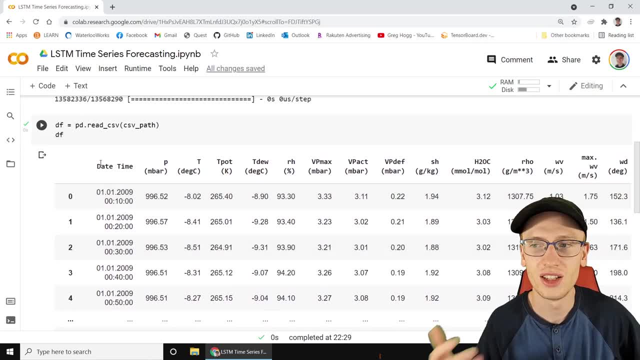 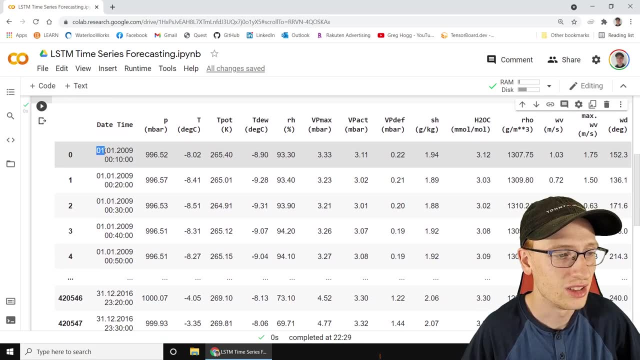 going to zoom out for a brief moment just to show you this, but I'll zoom back in shortly. It's a very big data set and I don't want to bore you with all of it, but basically the important part is that this is the day of the year, the day of the month, or basically not the day of the month. the month. 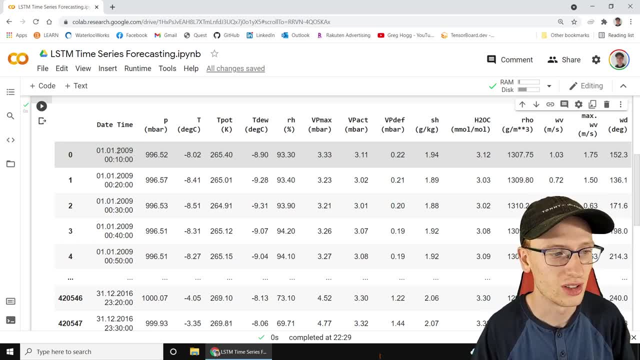 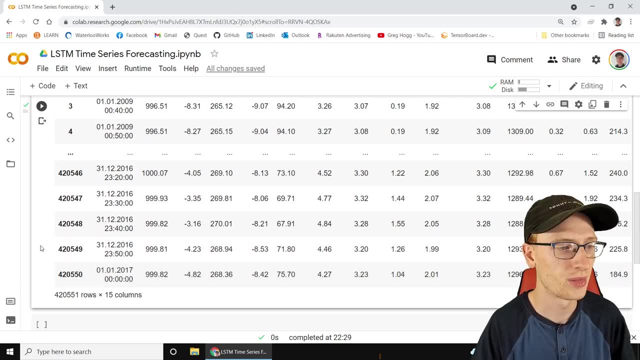 itself. So this is going to go from zero one up to thirty one. This one's going to go from zero one up to twelve and 2009, we can see. in the end, that goes up until 2017.. Okay, I guess the very beginning. 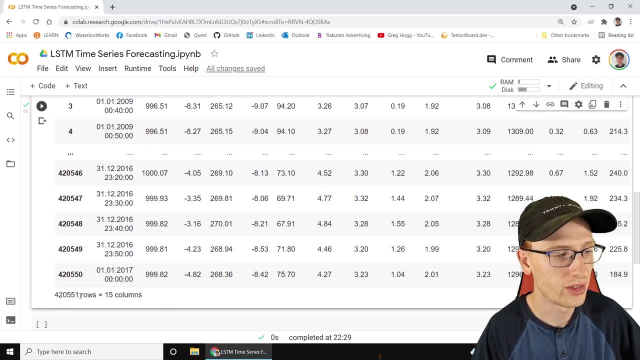 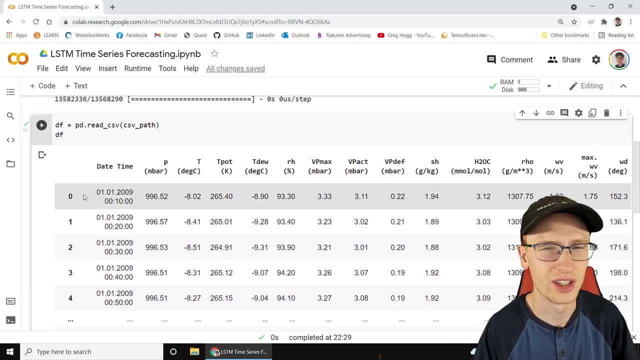 of 2017, so the end of 2016.. We have quite a bit of information here: 420,000 rows. So basically, this is all of these climate measurements in a particular area, it doesn't really matter where, for 10 minute intervals. So that's that makes sense why we have so many of these things. We have 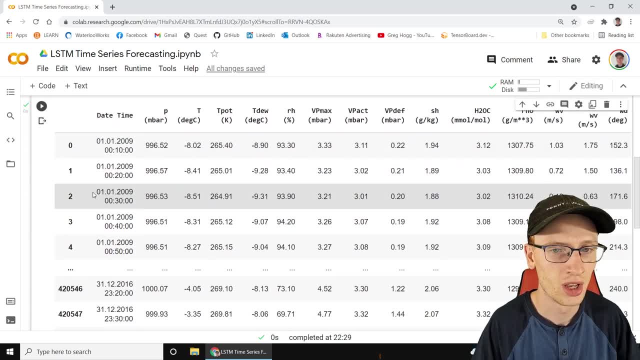 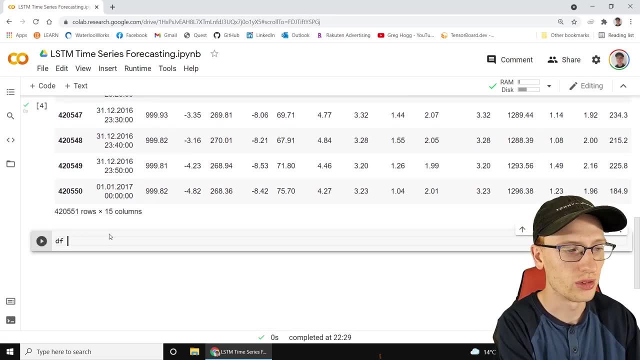 literally every 10 minutes for like ten, eight years or so. So we don't really want that much. I mean maybe for for your use case. if you're going to spin off this, then you might, but we don't really want that much. So I'm going to show you how to take way less than that We're going to do. df is df. 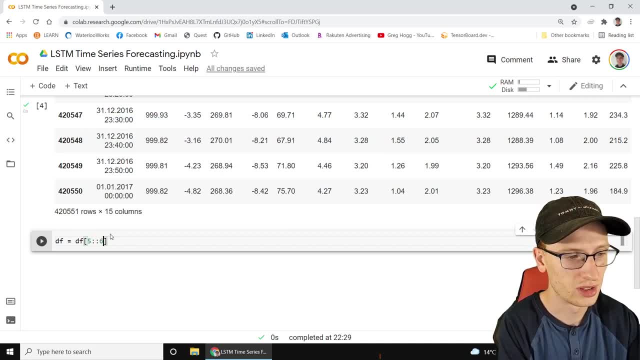 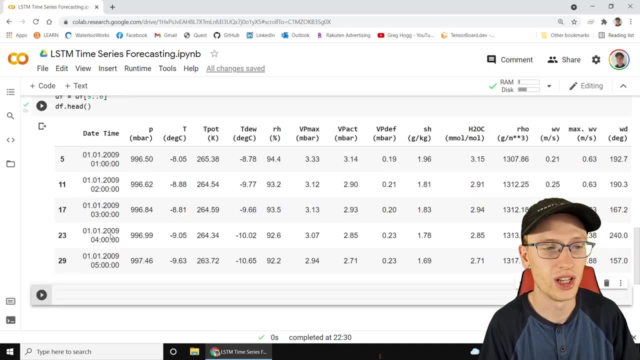 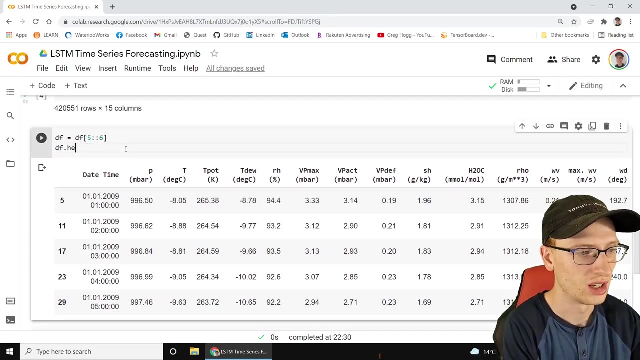 five. so starting from five, and then if we do the double colon that says take every sixth only, And if we're, if we mean take every sixth, well, if we have 10 minute intervals, this is really saying, you know, take every hour instead. So here is dfhead, and if you really want to see a little bit, 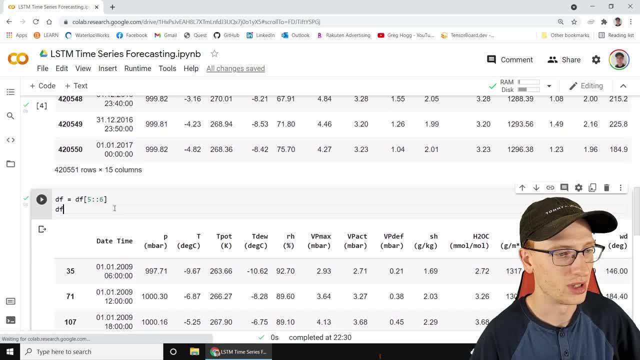 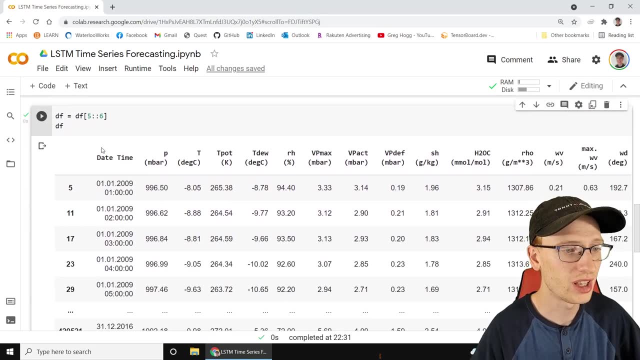 more than that, Go ahead. but actually that ruins it because you can't really call this twice. So I do have to call that, run it from back from the beginning if I want to do that. But yeah, we have this huge data frame which now we have every hour. So it's one, one o'clock, two o'clock, three o'clock and that's. 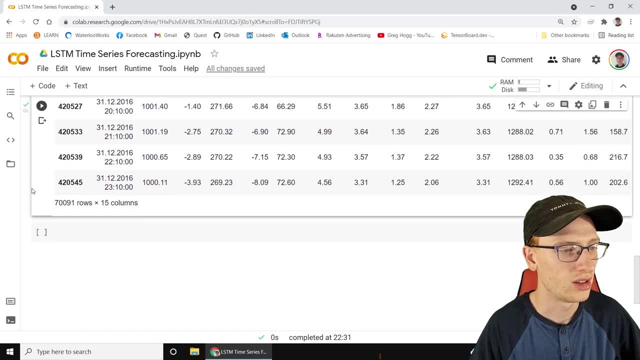 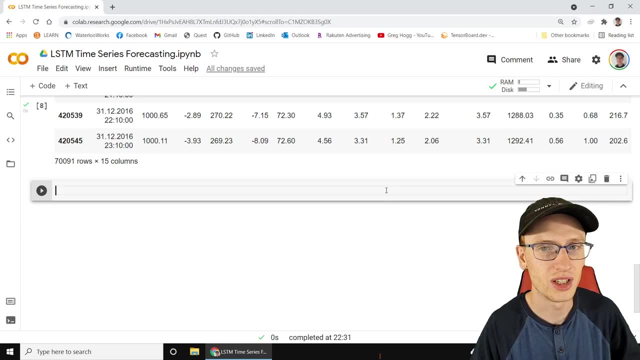 going to start from the morning, So this is 24 hours clock And, yeah, so we have 70,000 rows of data here which are going to be very useful to us. And, just so we can plot this a little bit easier, I'm going to be doing something involving dates, and dates are always going to be a little bit more. 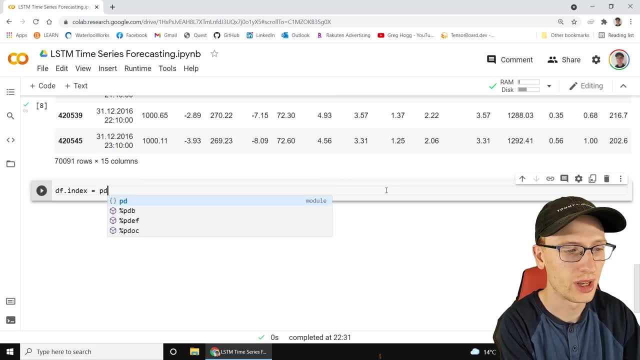 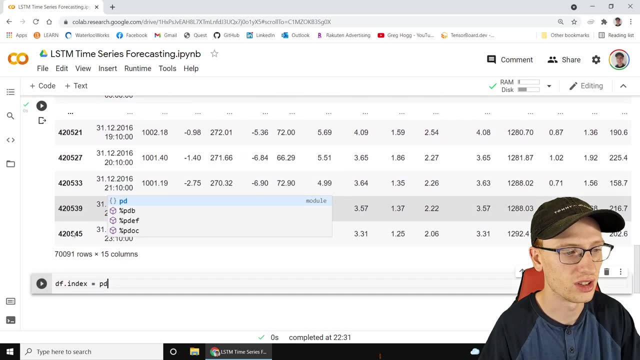 weird, So I don't really want to dwell on this too much. But we're going to be using pandas date time function, So we'll set the index, which is going to be basically this column right here. The first one is the index. here We're going to be setting this index equal to the pandas dot. 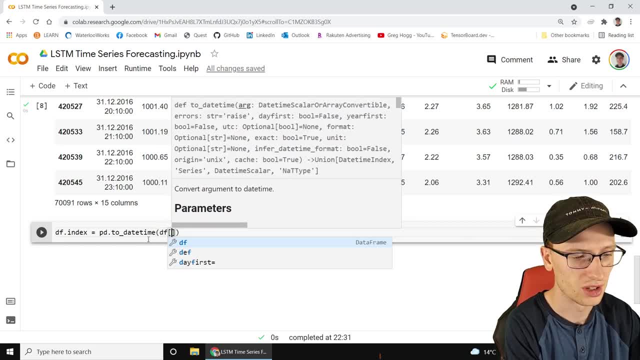 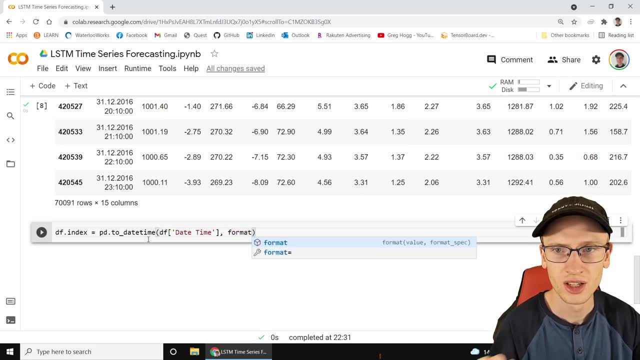 two: date time of df, sub date time. Okay, luckily collab grabs those names for us, right like that, And then we can get the format is equal to. I again don't really want to bore you with what this is in particular, but at least with typing it we can see that basically we're saying the format. 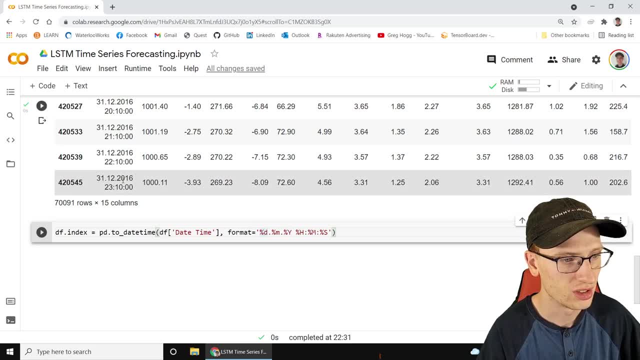 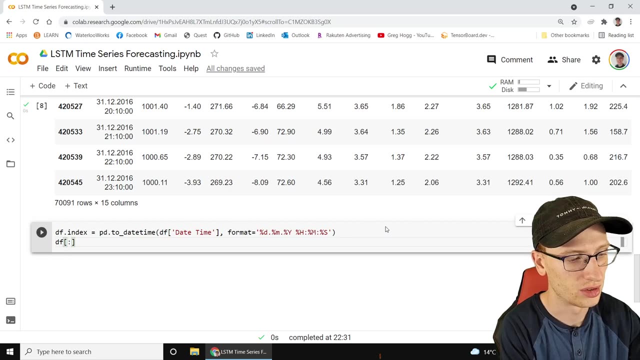 is the day dot, so the day dot the month dot the year, and then there's a space, I guess, and then hour, month, second. Okay, so that's the, that's the format of the data, and if I do something like say I'm going to, I'm going to purposely grab like a particular day, just say the first day up until. 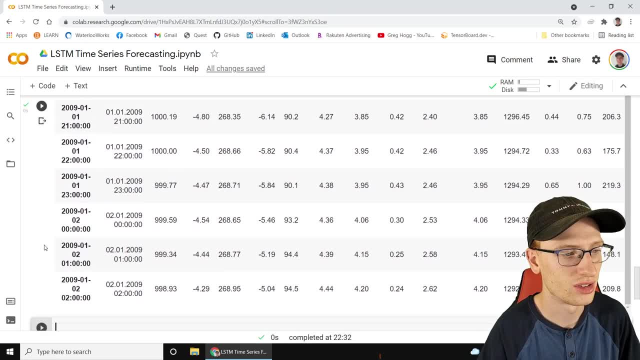 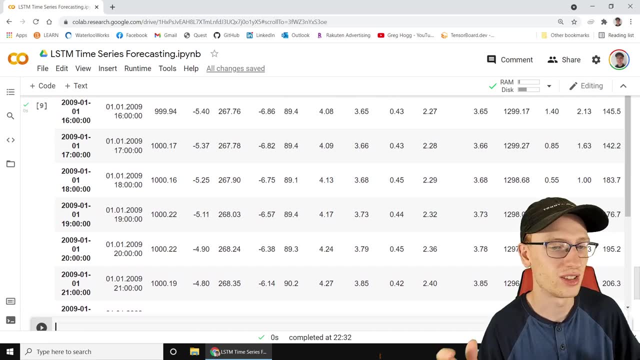 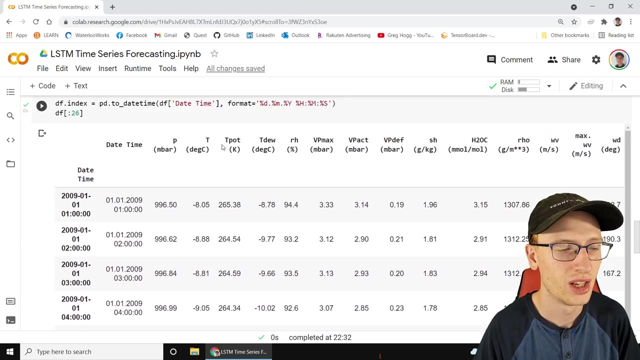 you know, 26. it's definitely that's going to be 26 hours. So the first 26 hours are right there, Okay, so so this is great, but this is very complicated and yes, absolutely you could. you could look at all these variables and say, okay, maybe make some complicated time series forecasting model. 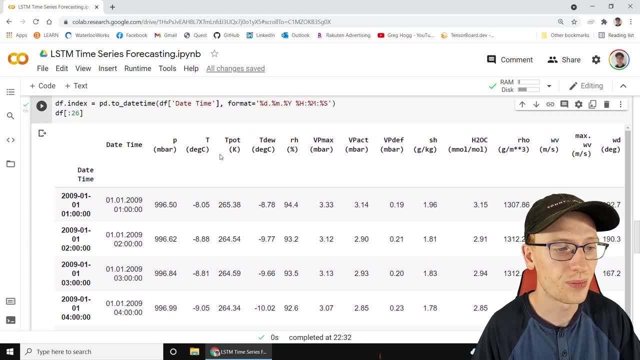 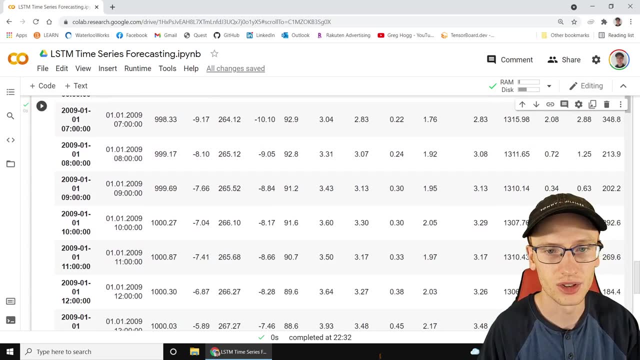 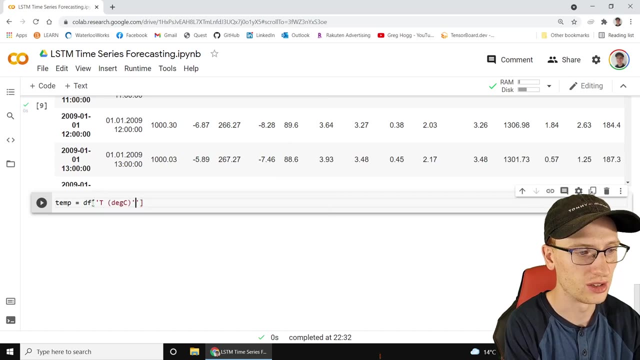 but we really don't want to do that. Here is t in degree c and we're going to focus in on that one right there. So basically we can grab that very easily. if I was to do something like make a variable called temp, Temp is equal to df sub, just grab that t degree c. 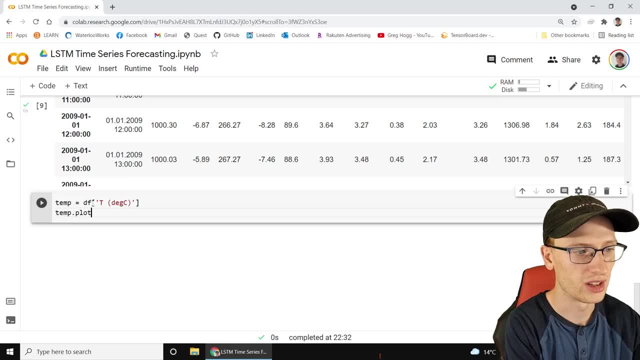 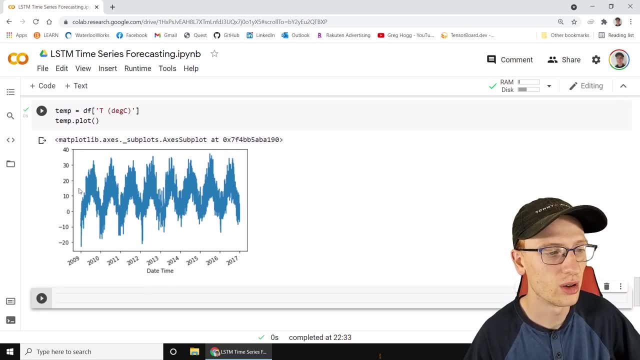 and I don't know why it always makes too many quotes. and we can plot it like this, and that's why I bothered to make the index to be this column, so that it knows that this is this date time where here, over years, clearly we have this recurrent pattern and it's not really. 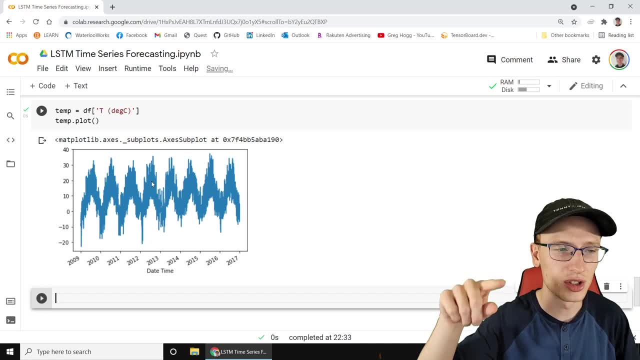 surprising We'd also have in a day. there's going to be fluctuations going up and down as well as per year. we know that each year it's going to. it's going to go up and down as well. So we're going to see that pattern and, yeah, we're going to. we're now going to make a little bit of a 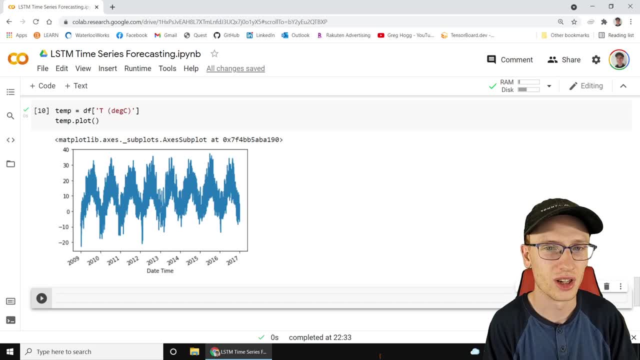 guess, using the method of interpolation, and we're going to try to find the right way to do that. So we're going to use this method and we're going to take it slow, and take it slow and slow, and take it slow and take it slow, And then we're going to use this method to try to get. 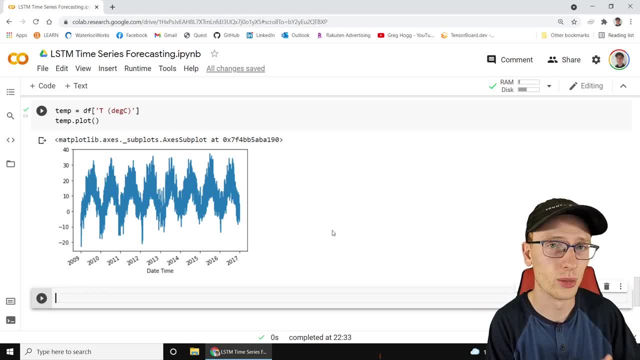 a very complicated function, So bear with me on this one. it's not too bad, but I want to take it nice and slow. So the idea is that for these deep learning models we need the data always to be in some sort of input matrix. at least, matrix is usually the term unless, unless it's more complicated. 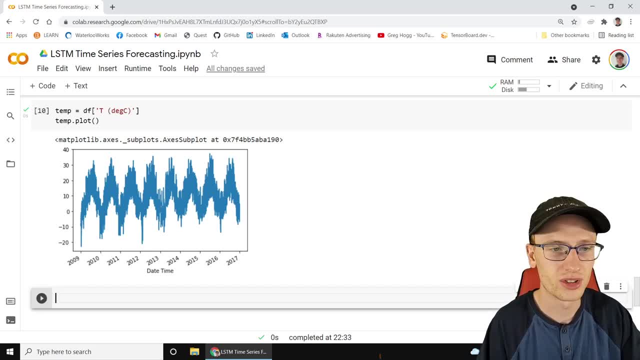 label. So what I mean by this is we're going to end up with something, And actually it's. it is going to be slightly more complicated than matrix, But basically for forecasting we need to look at, say, hey, the last five days or so For us actually we're going to use, since we have our 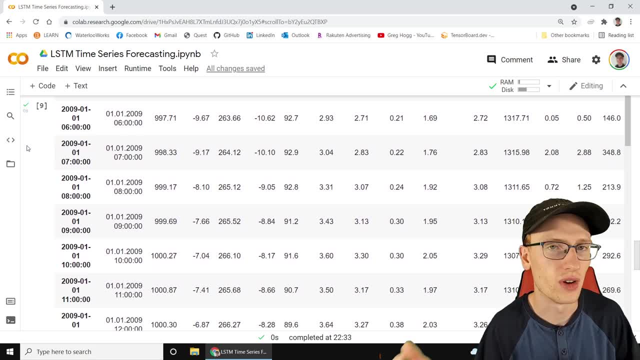 increments. we're going to say it every, maybe every five hours. we'll try to predict what the temperature is for the next hour. Okay, there's a lot of different choices here, But for forecasting model, a simple one that makes sense, where we look at, say okay, what was the temperature at? 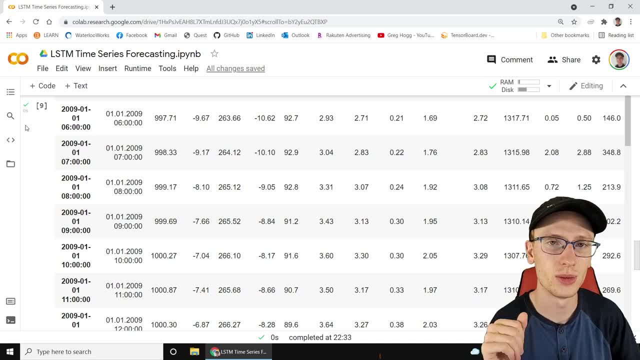 one o'clock, two o'clock, three o'clock, four o'clock and five o'clock. that's five different measurements, And then we'll try to predict what it is for the six o'clock one. And then, after we get that one, well, we would bump it over one step or we'd say, actually we don't care about one. 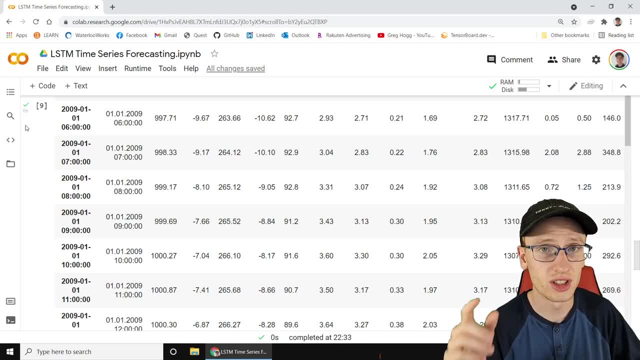 o'clock anymore. we'll take two o'clock, three o'clock, four o'clock, five o'clock, six o'clock. that's again another five, but we bumped over a step And the corresponding output is going to be what it was at seven o'clock. Okay, 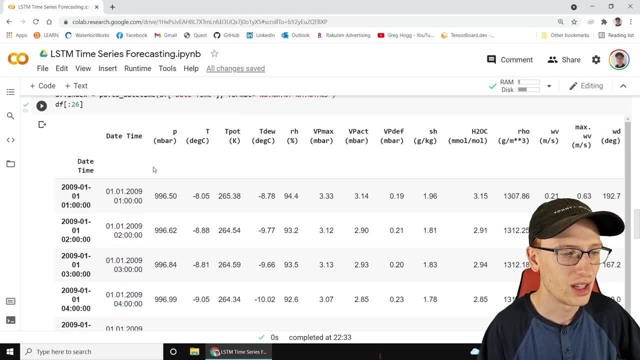 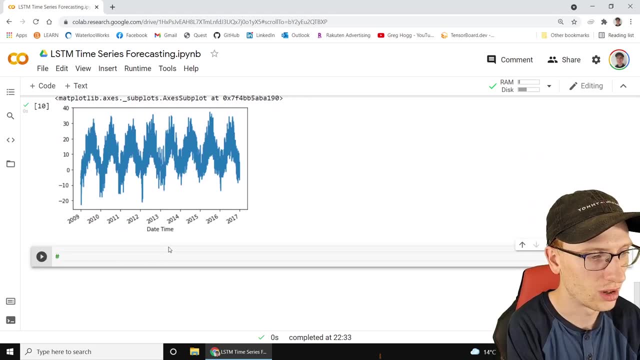 We're going to make this function where we we change this thing into this sort of other matrix that looks something like this And let me draw it out to you It's going to look. if I was to draw a comment, basically, it would look like this: where we had one o'clock, so the temperature at one. 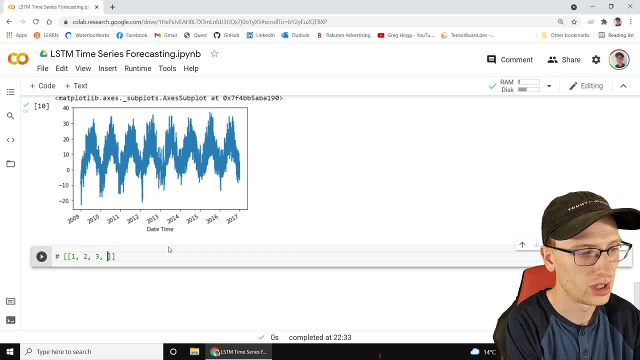 o'clock. I'll just do one for short: one, two, three, four, five, six, And that's going to be our first input And our corresponding output, for that is going to be what it is at, And actually. 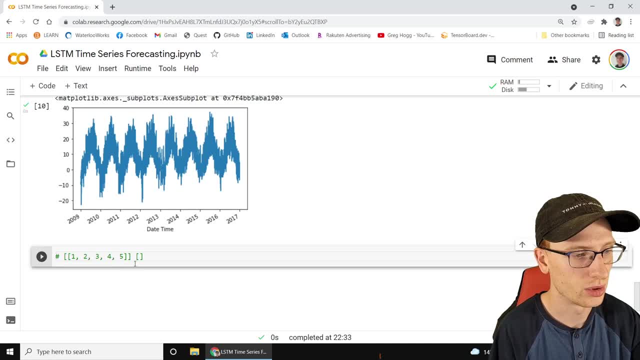 I said six. there, that's been. really. if I'm going to stay consistent, that should be one, two, three, four, five And then what it was at six o'clock. Okay, that's the corresponding output here. This thing I'm going to call x, this whole thing is x And this whole thing here is y. 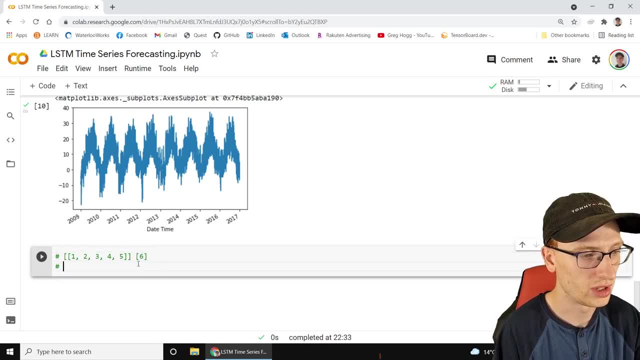 we're going to build this up, And then the second row of each of them. well, we bump it over one step And we'd say, okay, this is then two o'clock, three o'clock, four o'clock, five o'clock. 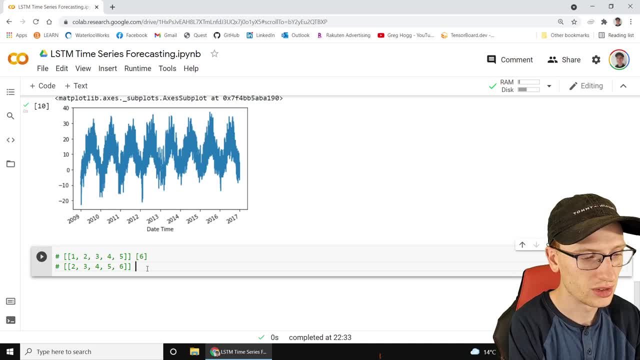 six o'clock And the corresponding output is going to be at seven. Okay, so you can see this kind of move down here, because after we saw these first five, we were guessing for this one. But now we've guessed for that one, And so we bump one step. 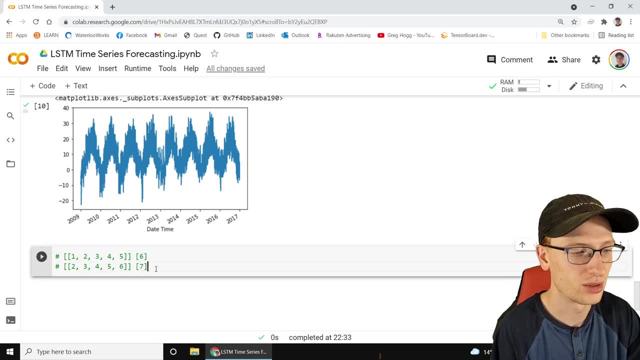 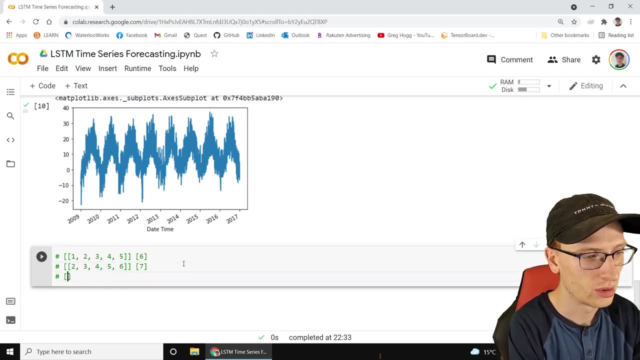 over and we'd include that into our input to try and predict the next one. So this big long thing that we're creating here is going to be our y vector, And let me just show you one more. So it's very clear we would have. the next one is going to be three, four, five, six, seven, And 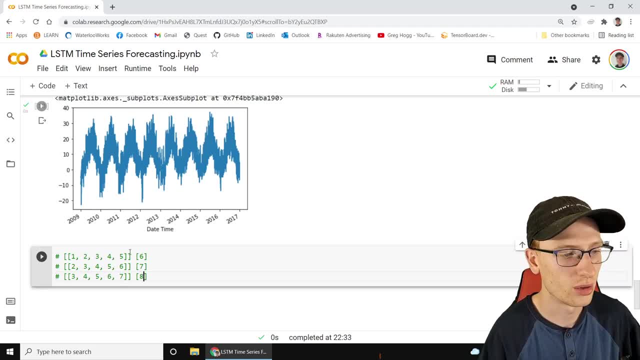 then the next one is going to be, and so on. we have to make this whole thing where this is our big x matrix And this is our big y vector, okay, where each of these are an input and this is the corresponding output. I know, I. 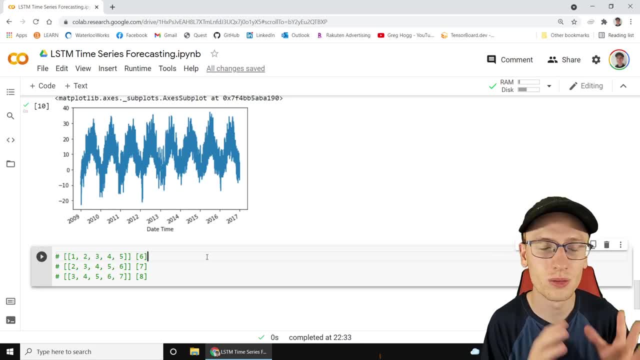 just talked about that for a long time, But that's really the whole super most important thing in this, other than just creating the model architecture of what's going on here. This is supervised learning: converting a forecasting problem to a supervised learning problem. 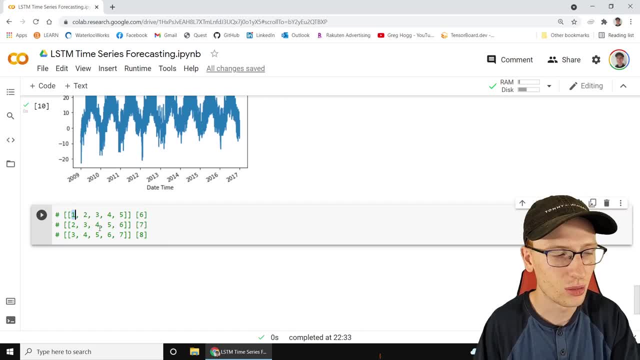 So we need to make this thing, And in fact we actually need to make this thing where we wrap each of them in a list. But it doesn't really matter, I can do that in the comments very quickly And as well in the code very quickly. 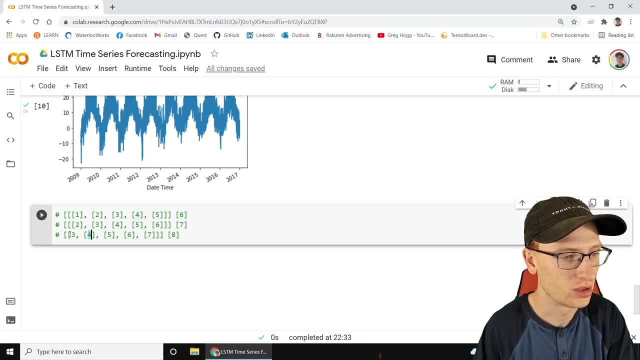 It's really not hard at all. You just wrap it in that Because essentially, if we were to do a multivariate, which means more variables, then you know, maybe we would include other sorts of variables in these lists as well, Like, maybe this would be temperature And this one would be. 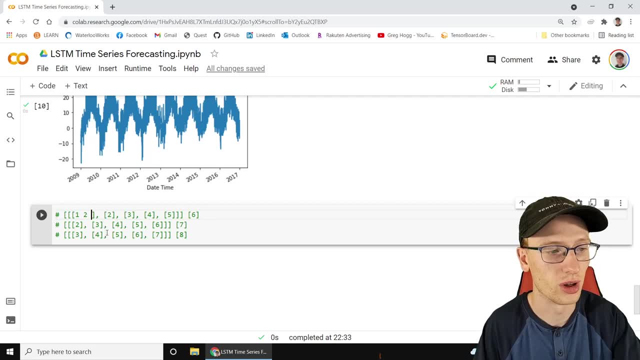 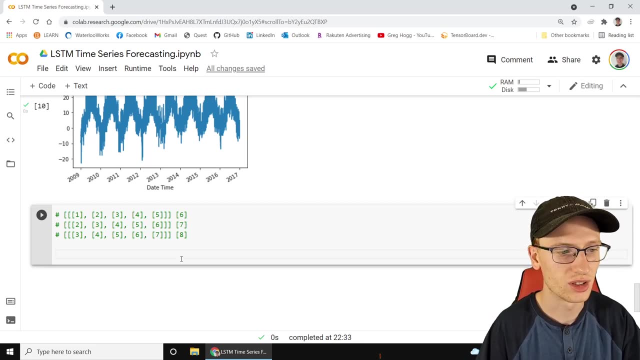 pressure, And this would be, you know, some other values, And then we would include other variables as well. But we're not going to do that, So don't worry about that. Let's create this function. So how do we do this? Well, we're going to call it to start. it's going to be called df to x- y. 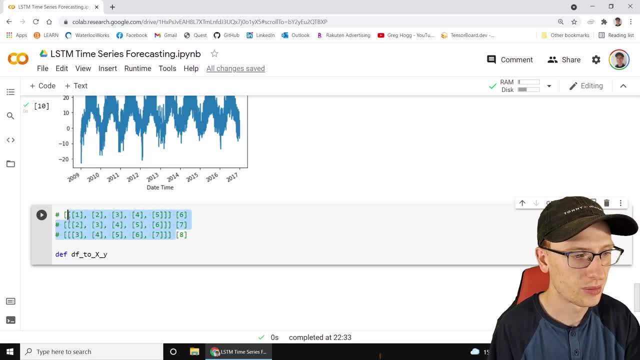 okay, or the x is going to be this input thing, This big matrix. it's really a 3d tensor, But it's. it really looks like a matrix. So define to x, y And we'll give it okay. df And. 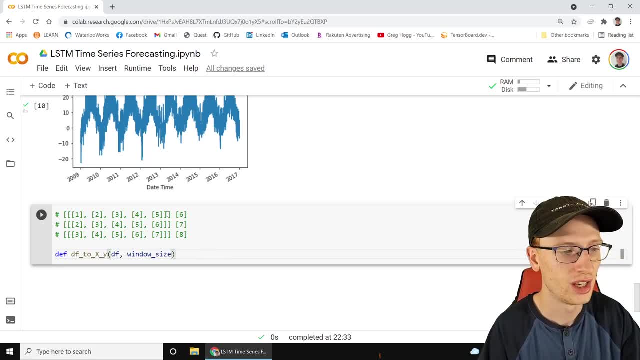 we're going to call it window size. Okay, what I mean by what I mean by window size is that we decided to take the last five, five measurements here, except we don't necessarily want this to be fixed in our code. we'll make it flexible, So we'll call the window size, And you know maybe. 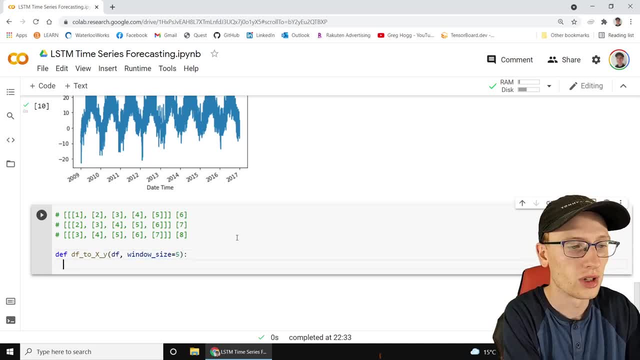 we'll just set it to be five for fun. So then, so that we're comfortable with that. Now we're going to quickly convert the, the data frame, to NumPy, So we'll do df, as NumPy is equal to df, dot to NumPy. 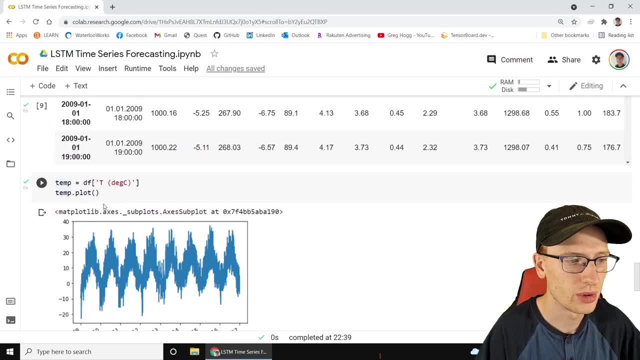 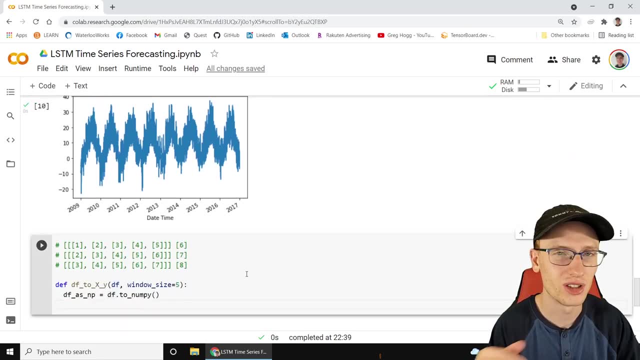 It's that easy And really the df we actually are probably going to call it with 10. And so that's just going to be converted to this long vector And that's totally fine. we got the values there so that we can kind of iterate over this thing in this weird window fashion to get the 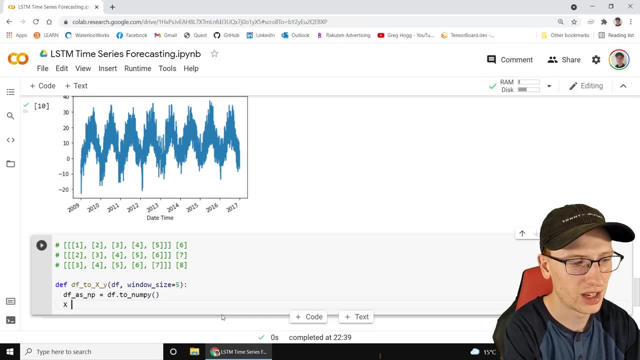 values. So, at one at a time, we're going to be building up this thing x, which is going to start out as a list, And we're going to be, one at a time, bumping it up with each of these, these rows. 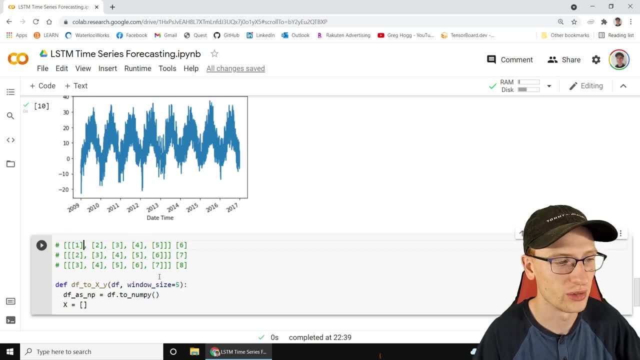 basically- and forget that these mini brackets are here- we'll deal with that shortly- But basically we have to add: this list of this is going to be like the first five values, And then we need to add to y, which is going to be this thing. we said y equal to this list as well, And 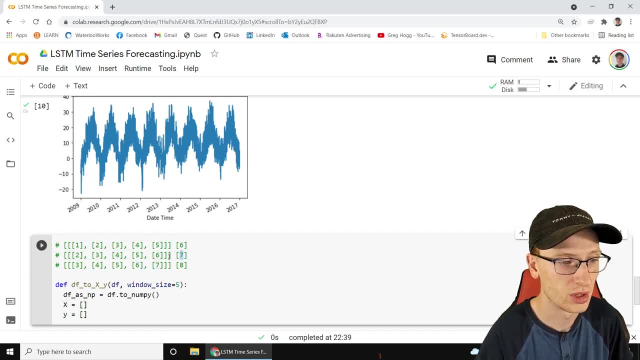 it's going to be this value And then we're going to append this value with to y, And then we'll append these values to x all at once. So we're going to be going through adding, say this thing, and to x, and then this to y, adding this all to x, and then this to y, and so on till we got the. 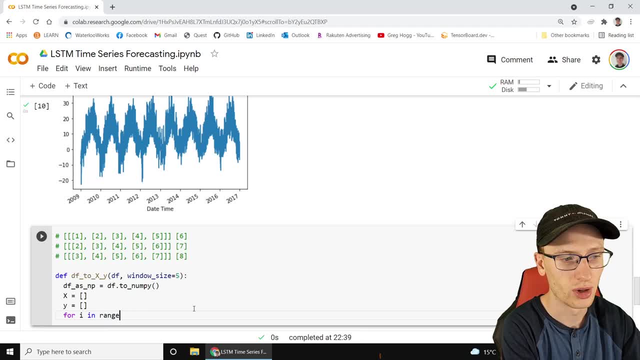 whole thing. So to do that, we'll do for i in the range of the length of DF as NumPy. Okay, so we're just going through, going through this thing within an index. that's pretty standard And we'll actually find later. 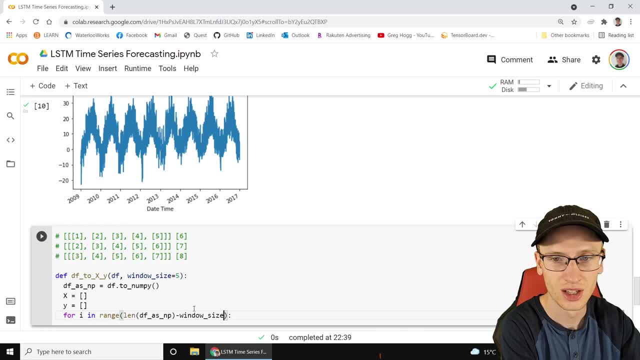 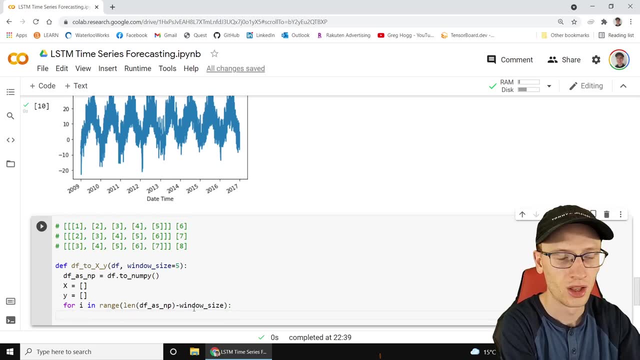 that we're going to have an error unless we do minus the window size, Because basically we'd start to get out of bounds. you could, you could really look into it if you wanted to, but it's not a big deal, And then we could do x, dot, append with what? Well? 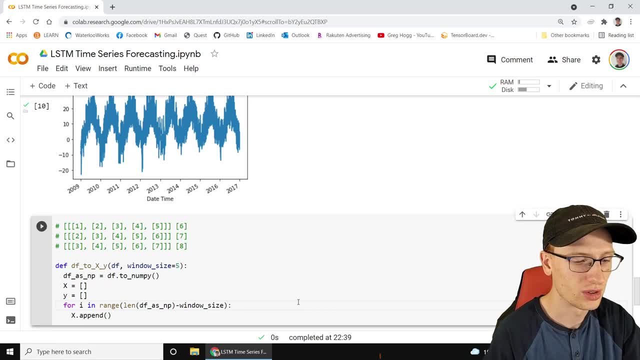 we need to add a value. So what we're going to do is we're going to add in this row thing And let me just grab this row first in a different variable, But this row is going to be first. let me just show you it's going. 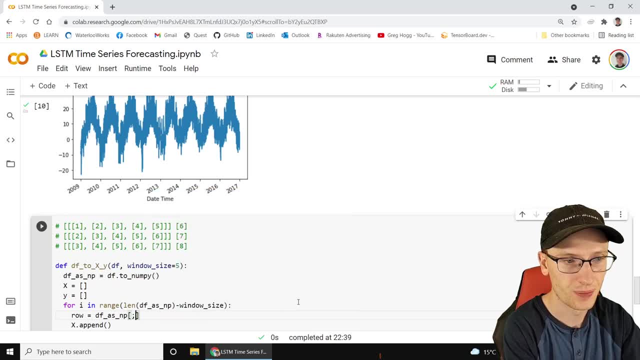 to be DF. DF as NumPy for with i okay, with i, from or from i until i plus five okay. So what that does is says: Okay, whatever I is right now, take just the next wasn't including it. and then 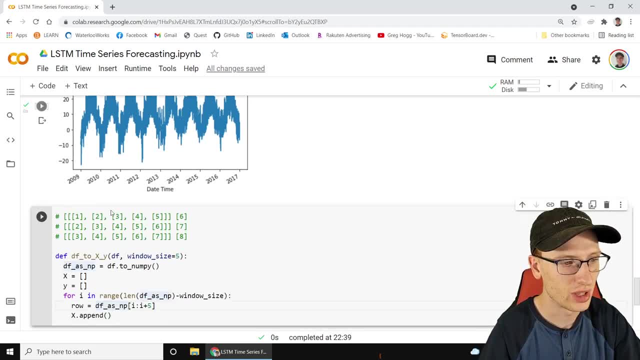 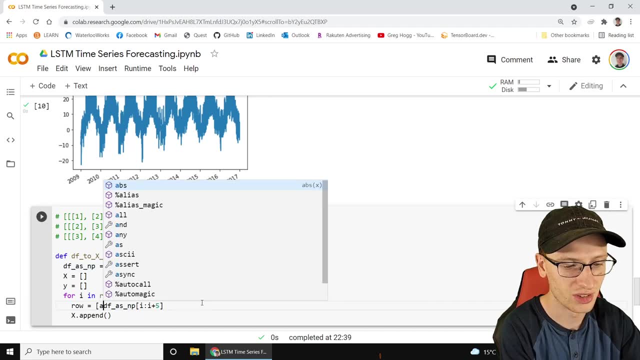 the next four, so really five values. And then to get in this extra little format here when we need the brackets, we can do a little trick here where we can just say the list of the list of a, four, a in this thing, okay. So that just wraps. 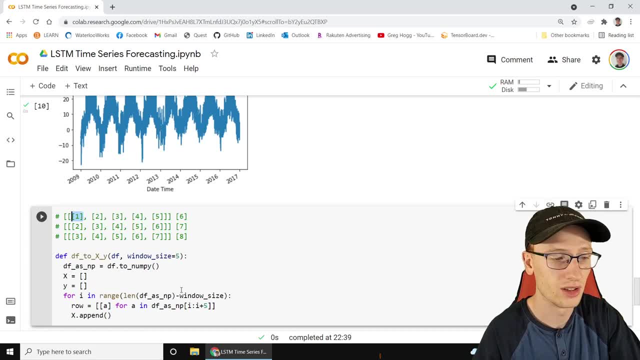 each of those values into one of these brackets, And and then that's just what the model is kind of like. it happens to like that input, Okay, and then we can append the row, And we can also append into y Well, the label. 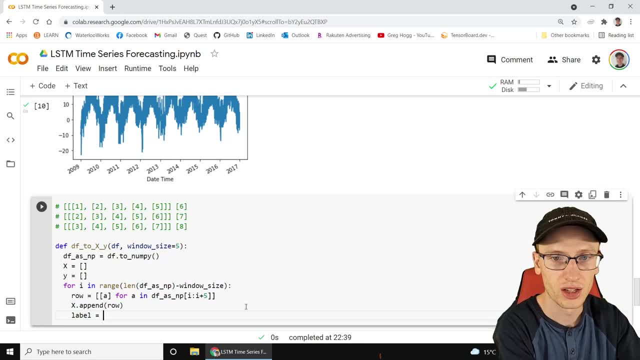 I like to call it the label. It's the true actual value for the input for that input row, and that label is going to be df as numpy sub: i plus 5.. Okay, so this thing, this member, doesn't include i plus 5.. It's going to be just the first 5, and then after that it's going to include the next. 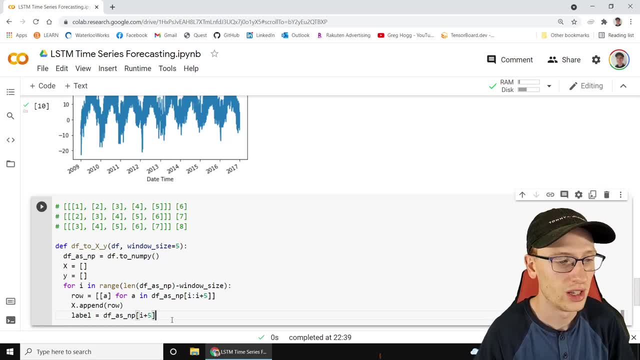 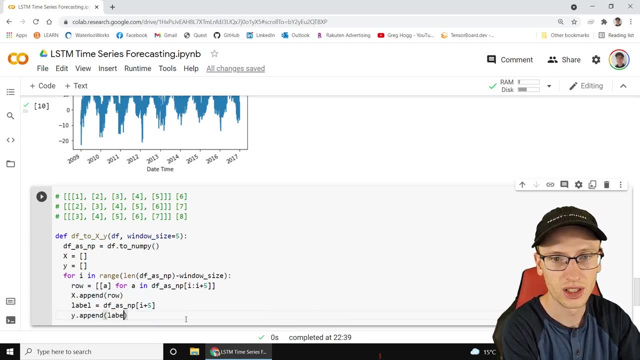 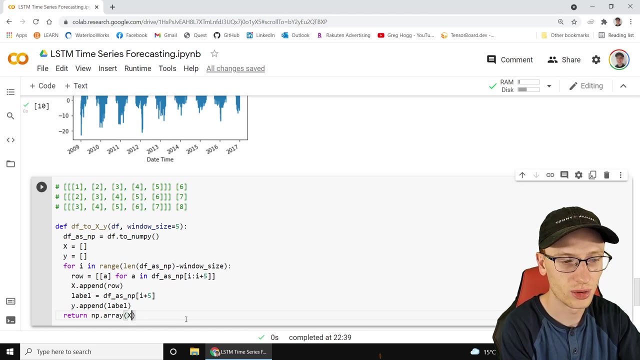 one here. If you actually say just this, i plus 5, it'll be the next one over. Okay, and then we can append the label with y dot, append the label and we can return, after all of this stuff, the numpy dot array. So I'm turning that weird list thing into a numpy array. That's important. We. 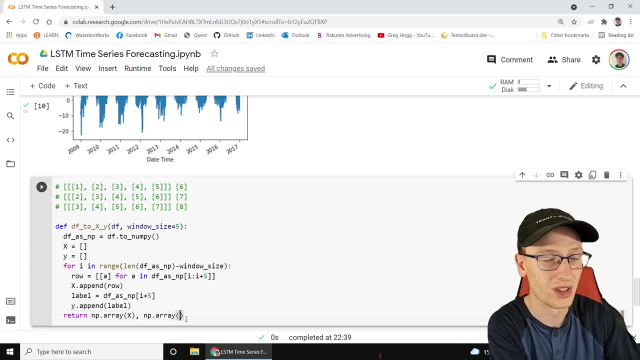 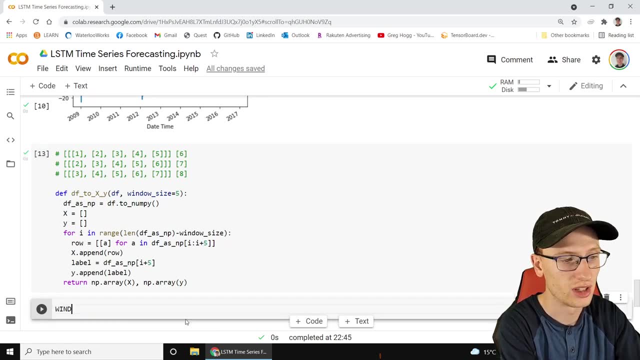 could have done it later, but I want to do it now. We'll return the tuple of the numpy array of x and the numpy array of y. Okay, and then how will we call this thing? We can set, say, the window. 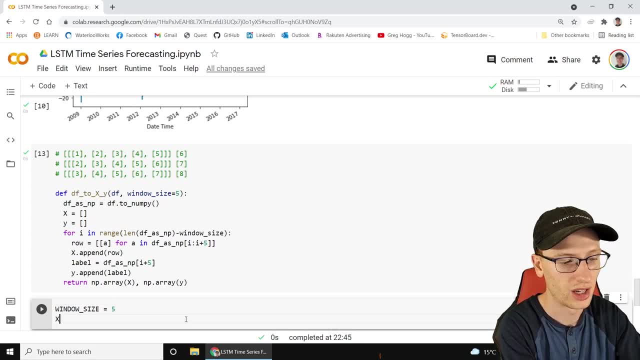 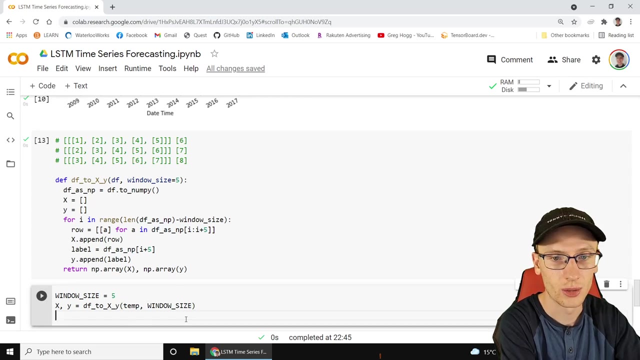 size equal to maybe 5.. We can set x and y equal to df To x- y. that's our function. with something, let's make it say temp. Okay, that's easiest right now. That's what we're going to stick with, and we'll give it the window size. Okay, and now? 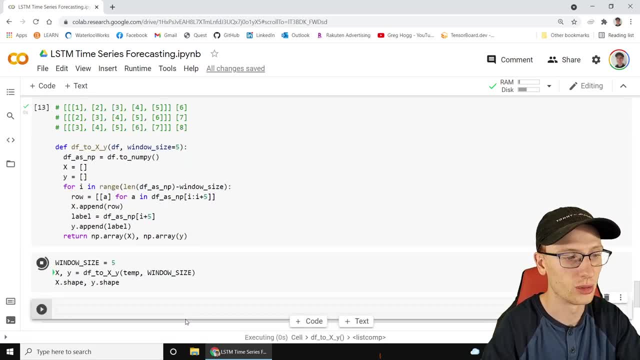 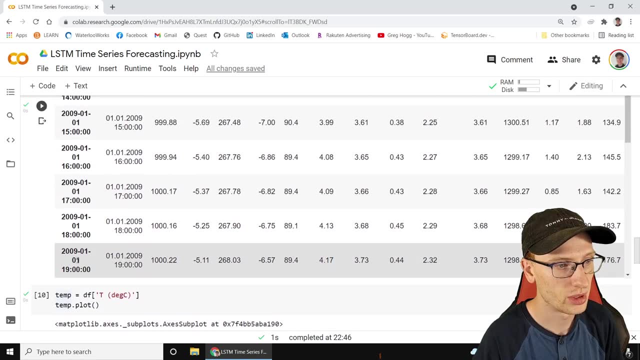 we can say x dot shape. I always like to output shapes so that we can see what we're doing: x dot shape and y dot shape. we can see we have 70,086.. Does that make sense? Well, we have up. 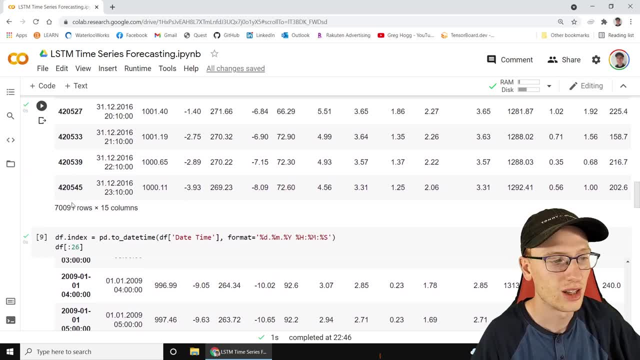 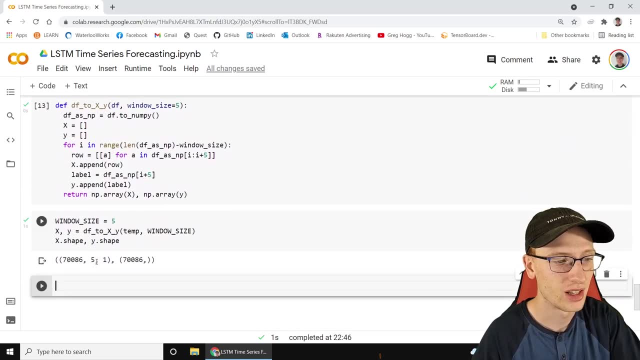 here. did we ever actually see there 7,091.. That kind of makes sense that we're missing 5 there. Don't think too much about it. But if you really want to drill down, this does make sense: 70,086,, 5 by 1.. Okay, and if you really 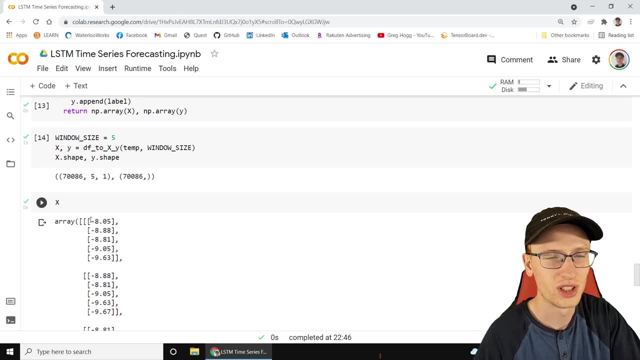 want to see it. basically it's this thing where it's printed in a worse format, the exact same thing in comments that I wrote out here, And then there's the corresponding label as well. If we go down to ask what y is, then y is going to be just each of the values and we don't have to wrap. 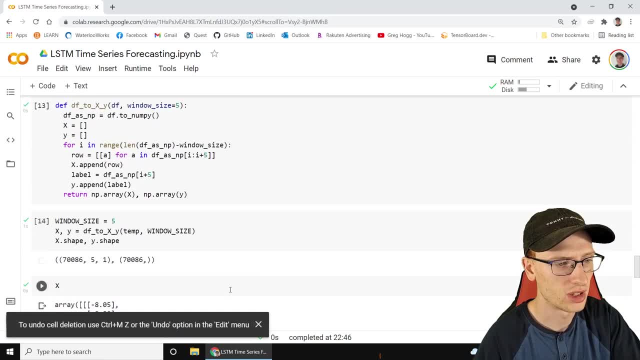 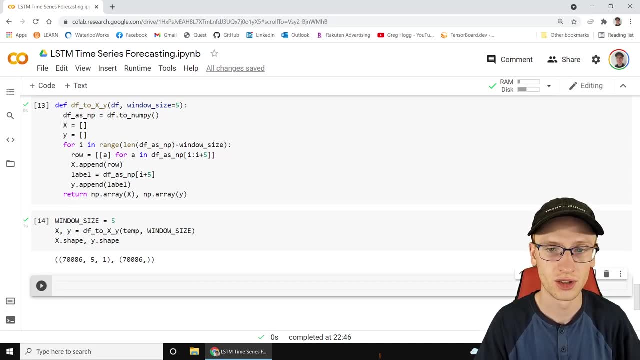 those in brackets. That's totally fine. Okay, I'm going to delete those cells because we don't really need them. And now we are ready to split this into train tests and validation sets. You know you want to train the model on some data. we want to validate it to make sure that it's actually being able to. 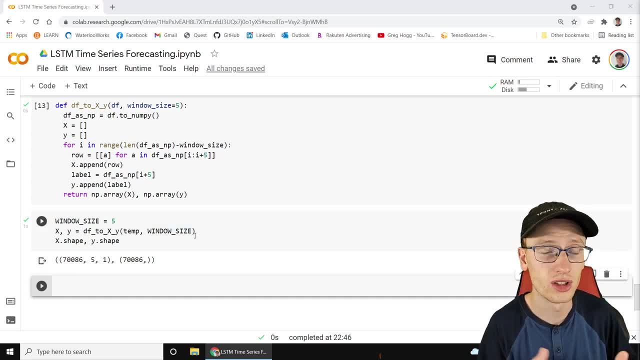 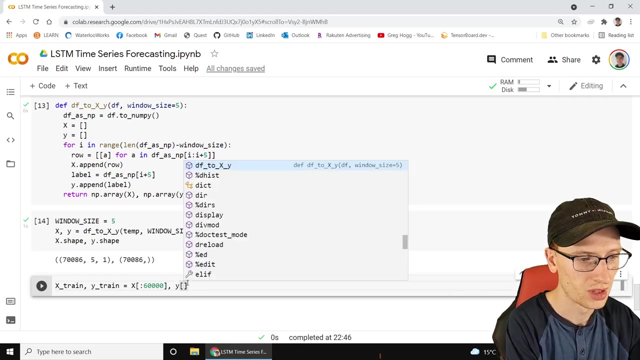 generalize and predict on new information. Another split into a test set. we'll say x train and y train is equal to. we're just going to split this in order here: x from 60,000, like that, and y sub y sub 60,000.. 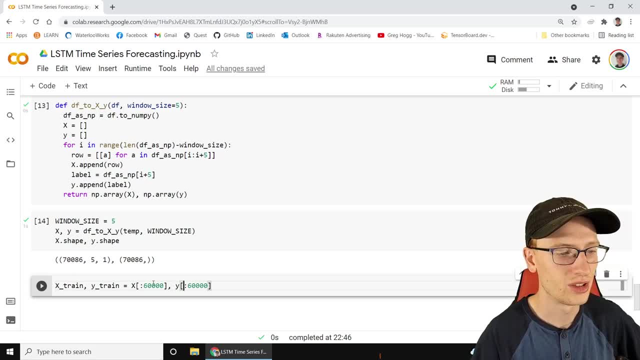 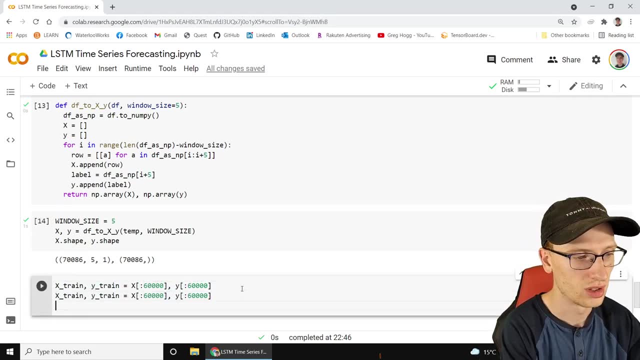 With the index there, with the colon there. So basically that says the first 60,000 rows. that makes sense with 70,086.. There we can change this to all changes to test and Val. this is going to be Val and that's going to be Val. that's going to be test and that's going to be test. Okay. 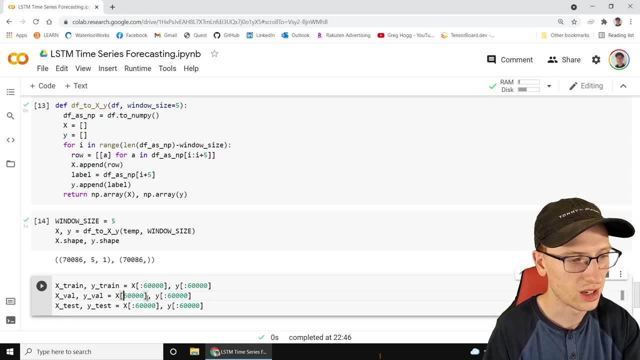 so here we're going to switch this to maybe say 60,000, up until 65,000.. And again, same sort of indexing in there will work just fine. And finally we can just say the rest: okay, give the. 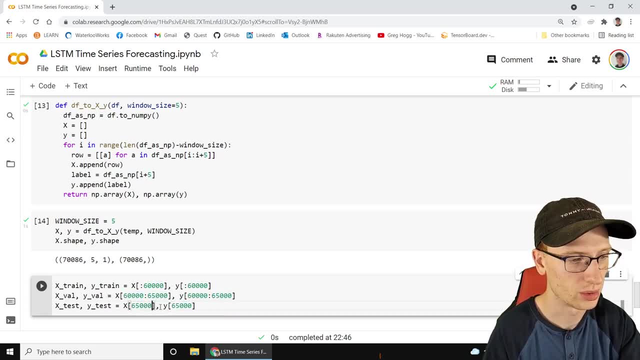 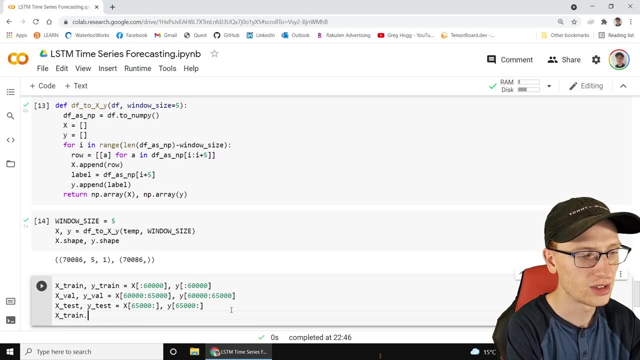 rest to test that rhymes. that's perfect. We're going to put the colon at the end there, splitting the data up like that. And again, like always, I love to open the shapes of everything: x. train dot shape, y, train y, train dot shape. x. Val dot shape x. sorry, y, Val dot shape. 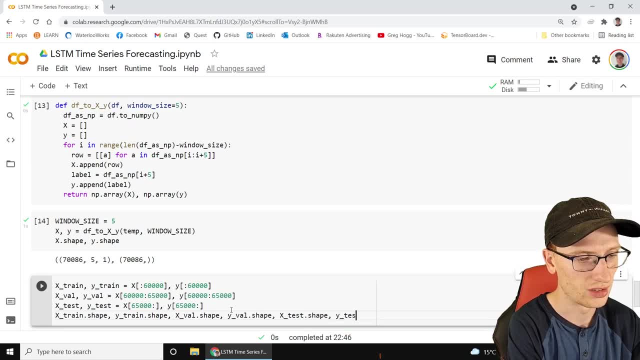 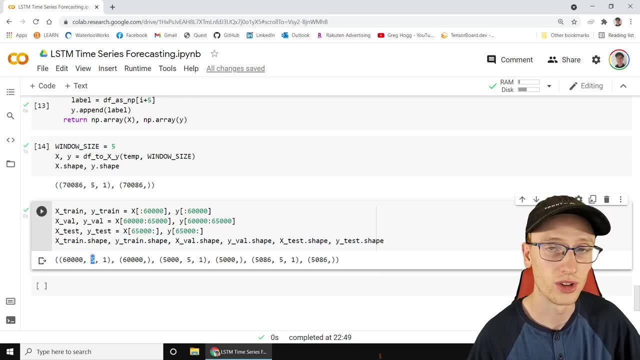 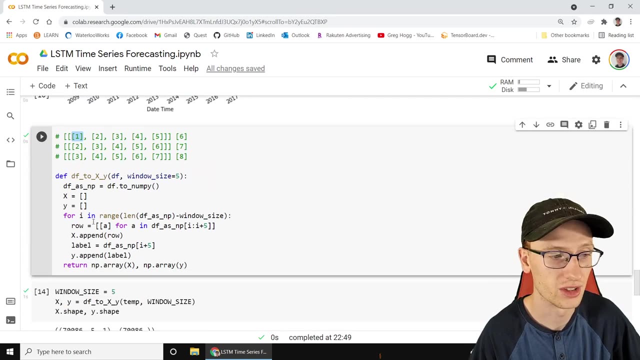 and x test dot shape and y test dot shape. the first 60,000 are for the training set it's. each of them are going to be five of the windows of five, And we're just going to be one here, which is why we it's, it's, we wrapped it in that little list here. it's just saying one. 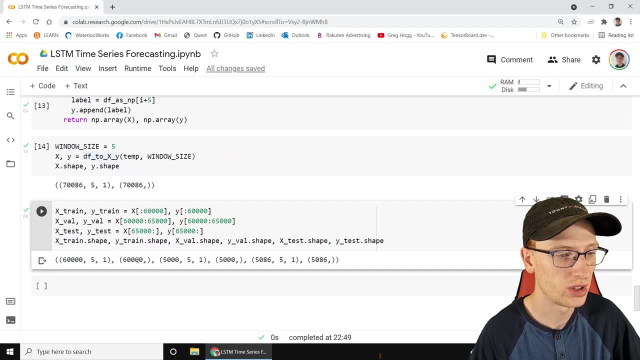 variable of interest. So we have 60,000 of this, this input, here, And then we have the labels. we have something very similar, but less for the validation and a little bit more, the last bit, for the test. Okay, so after that we are ready to compile our model And it's going to. 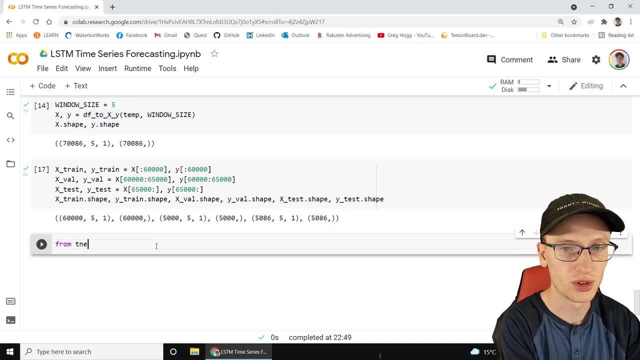 be training on this training set of information. So we're going to do a whole bunch of TensorFlow specific imports like tensor from TensorFlow, dot cures, dot models import or grits will get sequential. we will do from TensorFlow that cures dot layers. we're just going to import. 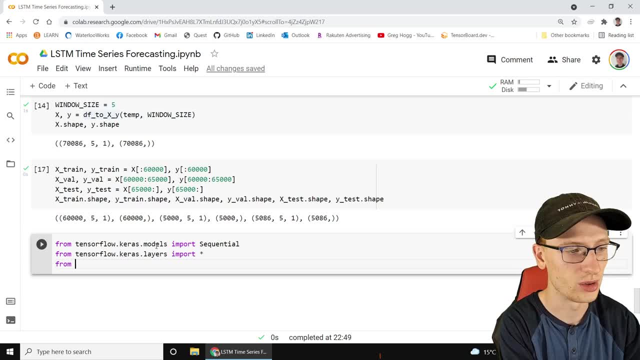 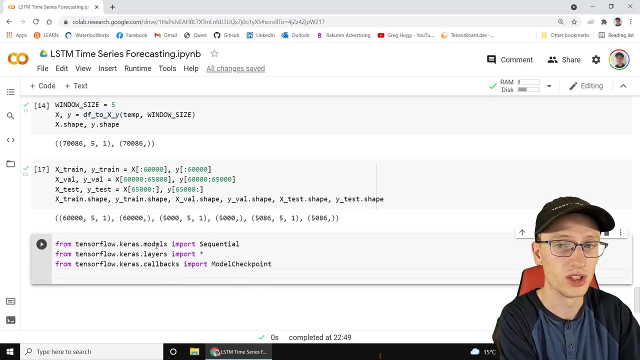 star to be lazy, But honestly, you know you can write them out, if you wanted to, from TensorFlow and tensor board. we don't need that. And TensorFlow dot cures dot layers- no, not layers. callbacks, import model checkpoints: this is for saving models. we're going to just save the model. 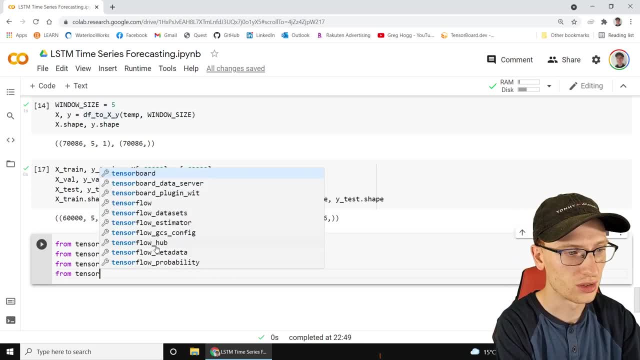 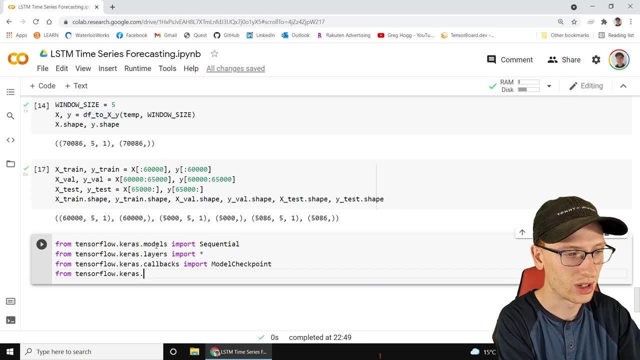 that does best. on the validation From TensorFlow: dot cures, dot callbacks, we want to import. No, I keep reading it wrong. I'm sorry for that. losses, import the mean squared error. Okay, so that that is for that makes sense. is our loss function basically So as the mean squared error? 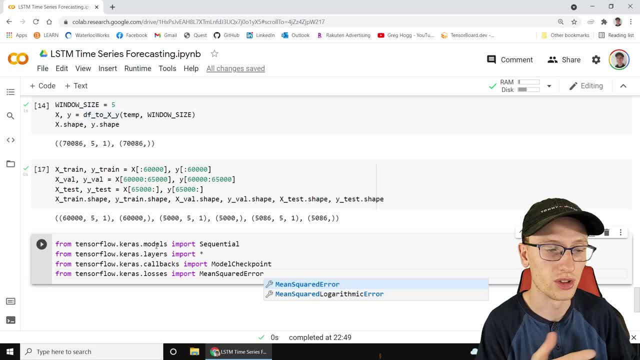 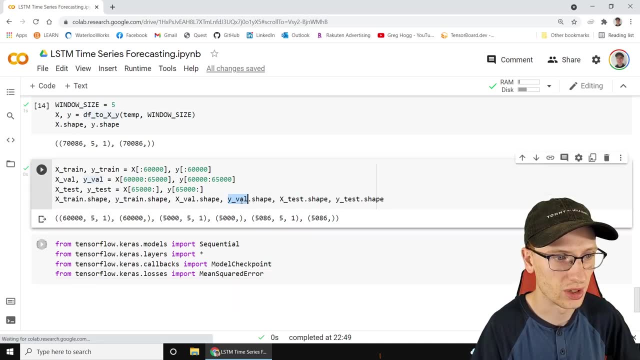 which is, you know, the. it is the mean squared error. we sum over the square distances between the actual value, which is that real temperature, that that label here, and what our model predicted. So if we sum, if we square the differences of those, we some all of them, and then we 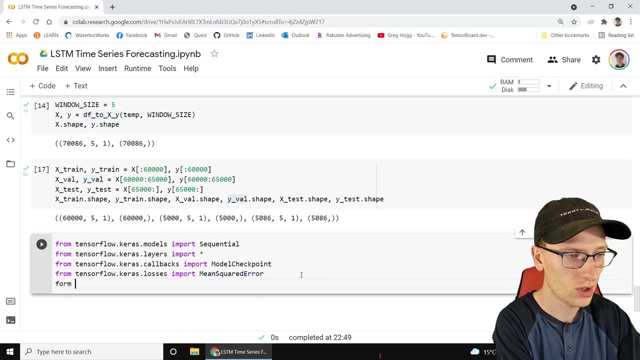 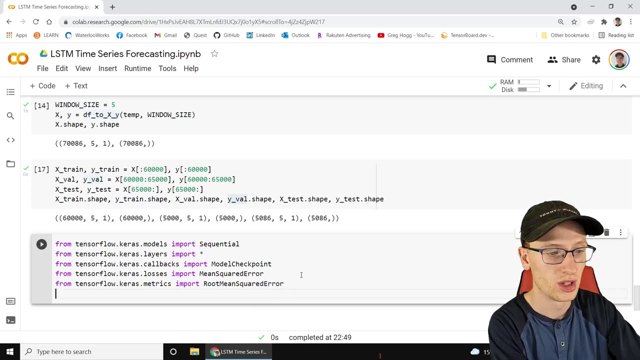 we take the average, that gives us the mean squared error. We don't really need this, But for fun we're going to output the tensorflowqrsmetrics import root mean squared error. Okay, so that's really just going to be the square root of the mean squared error there. 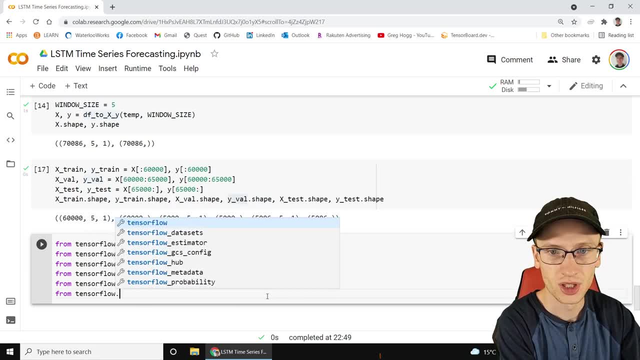 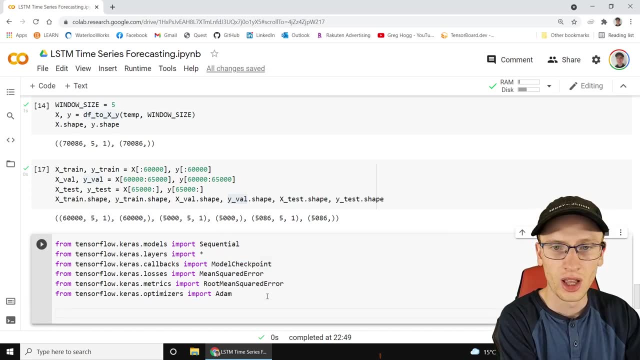 It's really just for us to look at, And then from tensorflowqrsoptimizers we're going to import Adam. Okay, and now let's make our model. So what do we want to do? We always make a sequential model like this: 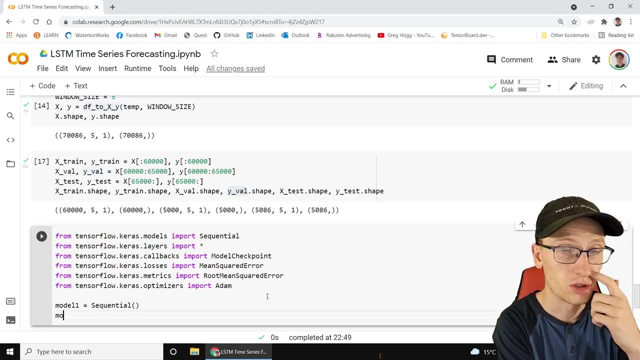 or at least generally, we use the sequential API. We are going to specify the inputs as usual. So model1.add input layer: Okay, we give it an input layer and specify the shape. It's going to be five by one, So this one, we generally ignore the batch. 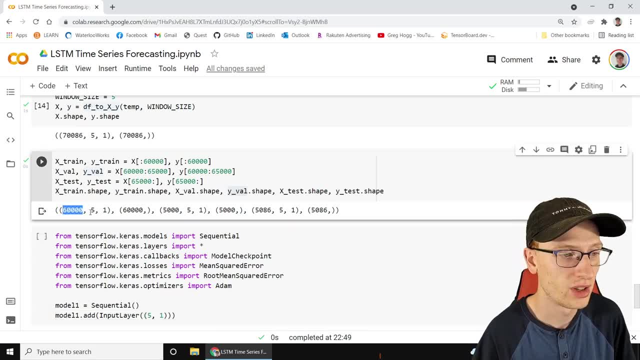 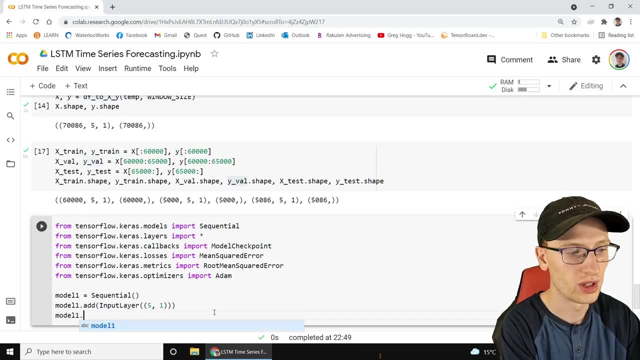 So this is the number of information that we have And then each of those, they are going to be a five by one vector pretty much. So we specify that there. And model1.add: here's where we do the LSTM. So we can do something simple and say: 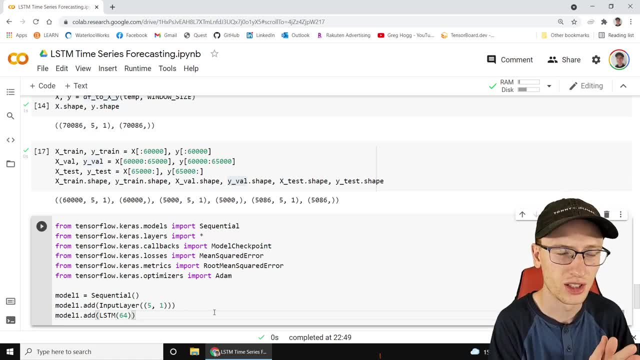 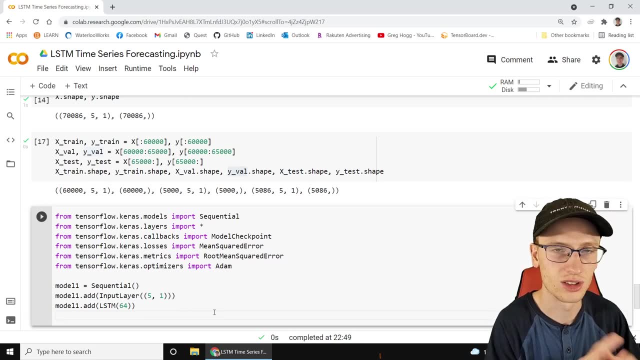 maybe 64 here. All right, I'm not going to explain all about the secrets of LSTM and the math behind it. I don't think it's that important For now. just know that you know we're going to pass this into this complex recurrent neural network here. 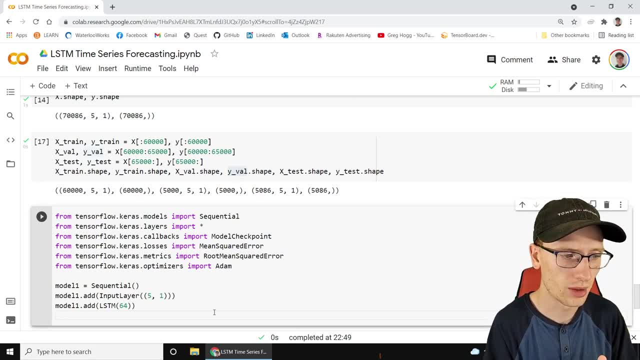 I mean complex is actually the most simple one there is really. You could also use GRU if you wanted to Look into that and play around with that if you want to, But that's what we're going to use today And we'll do- modeladd- model1.add- dense with eight and ReLU. 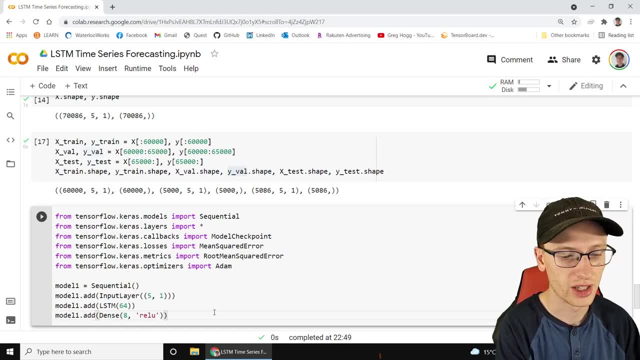 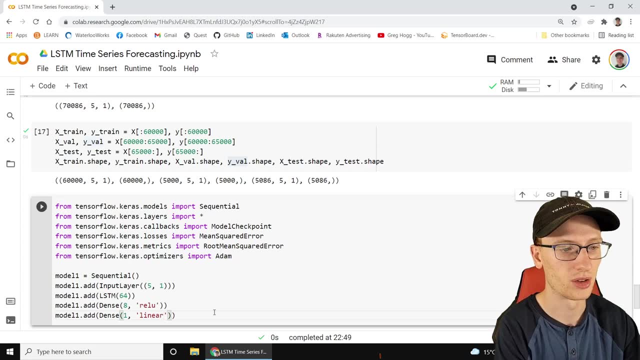 Okay, so after that we convert this to eight ReLUs And finally we have to make this model1.add dense with one and linear. Okay, we want a linear value. We're trying to predict some temperature, which is going to be a positive or negative value. 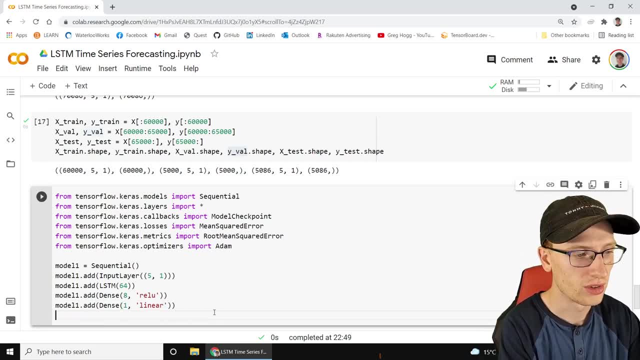 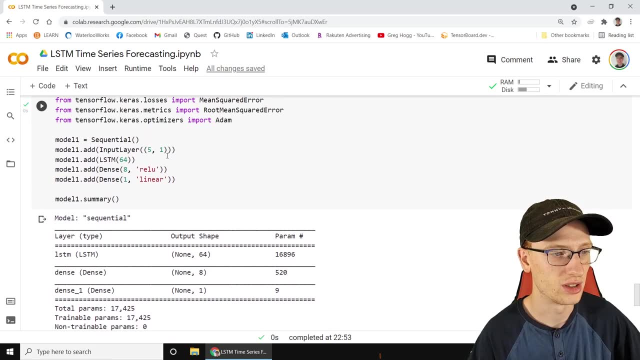 So we just want that to be linear. That's important. So finally, we can do model1.summary to make sure that everything works as we expected there And we can see: yes, it takes in a five by one. It turns it into this 64.. 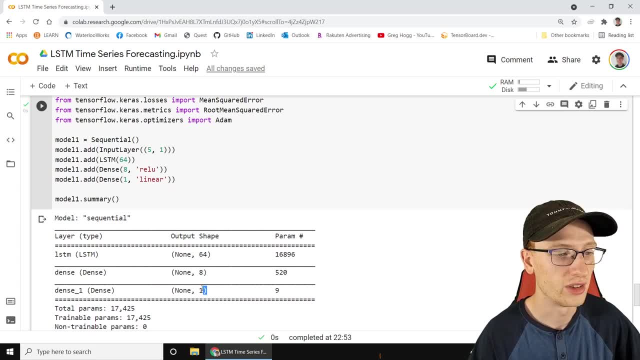 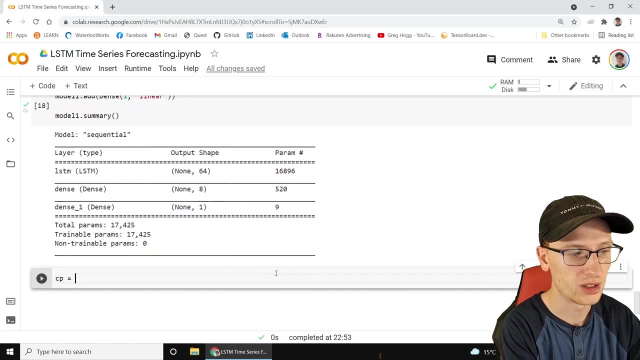 LSTM thing. We convert it to eight and then finally to one value at the very end. That's what's most important. Now, to specify our training callbacks we're going to do. cp is equal to model checkpoint. Model checkpoint with model slash- model1 slash. 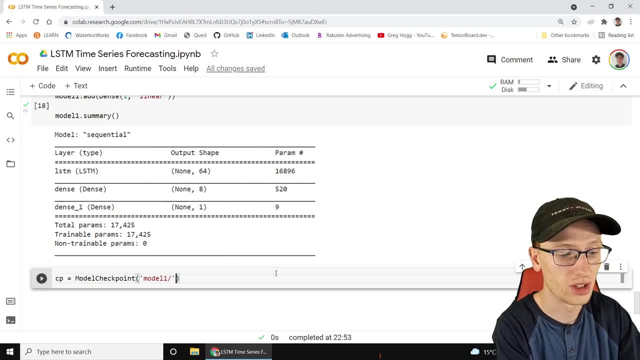 By the way, I'm saying model1, in case you wanted to go ahead and make different models. I'm really just going to stick with the one out of simplicity, but absolutely go ahead and make your own if you want it. What I just did here is set save best. 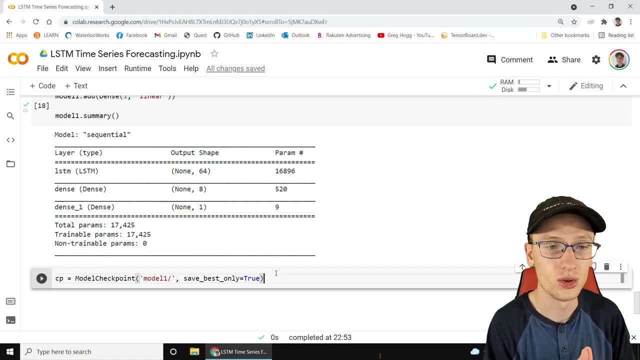 Only equal to true, which means I want to only well only save the best model, which is going to be defined automatically, by saying the one that has the lowest validation loss, which is really what we care about. the model predicting well on new, unseen information. 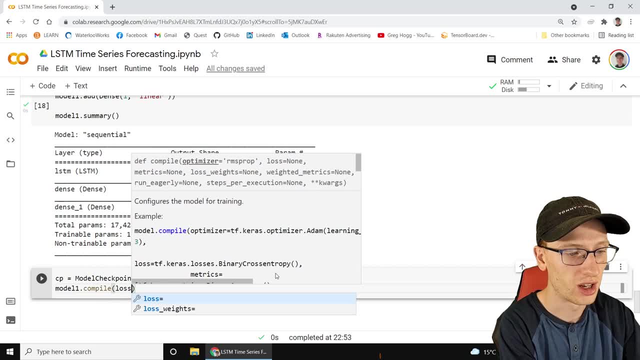 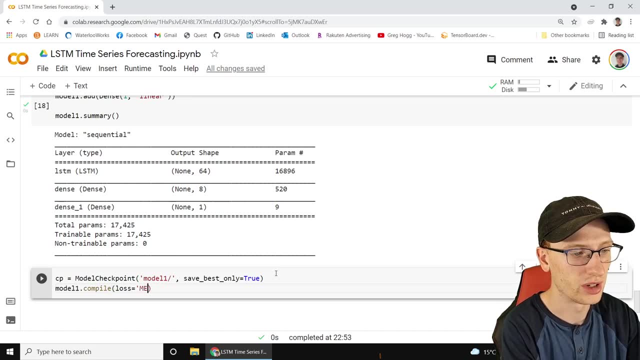 We will do. model1.compile with setting the loss equal to a short form for the mean squared error. His loss is MSE. I mean I guess, since we already imported it earlier, I should probably be doing I'd be doing: loss is equal to mean squared error, like that. 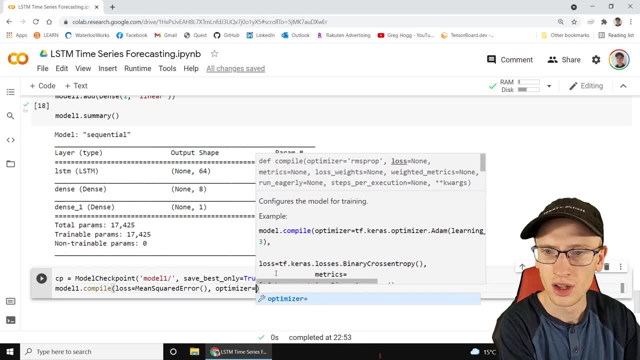 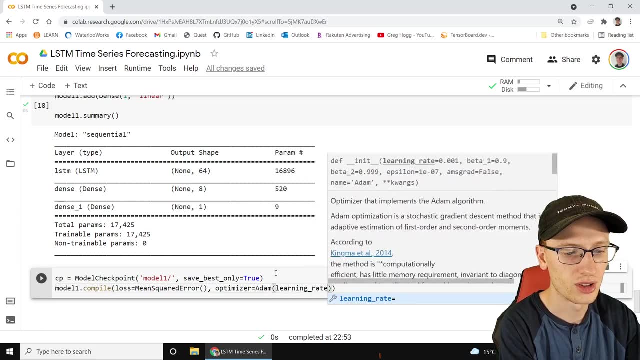 I suspect that'll work. if we error with that, That's fine Optimizer. Well, it's fine, but I'll change it. We're going to set the optimizer equal to Adam, with a small learning rate at first, And if you don't know what the learning rate is basically, 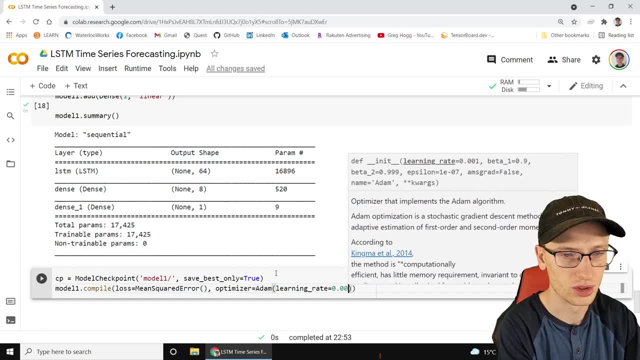 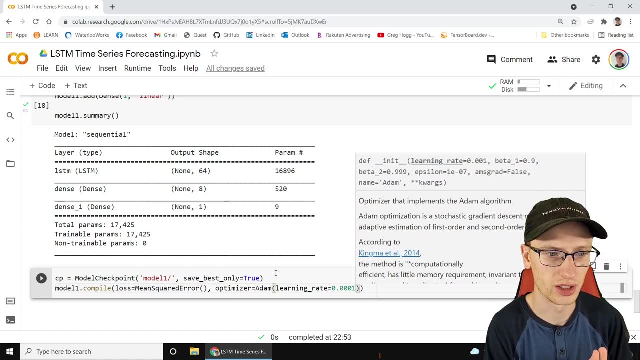 and I'm going to make this really small. actually 0.0001 actually make it nice and small. Basically, the higher this number is, the faster the model is going to try and decrease the loss, But we don't Want to decrease super, super quickly. 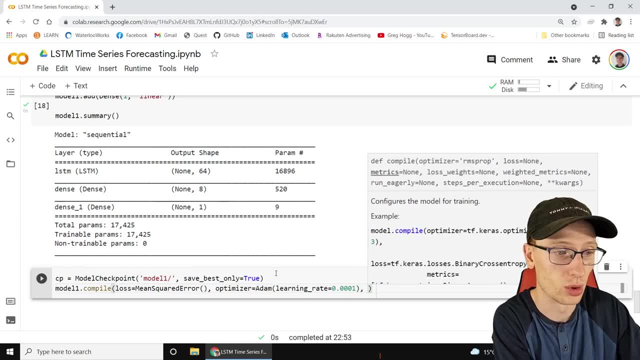 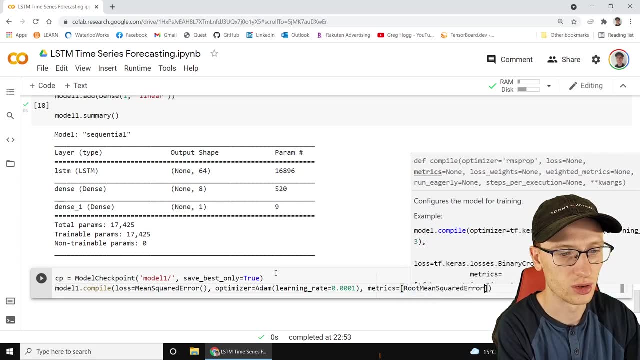 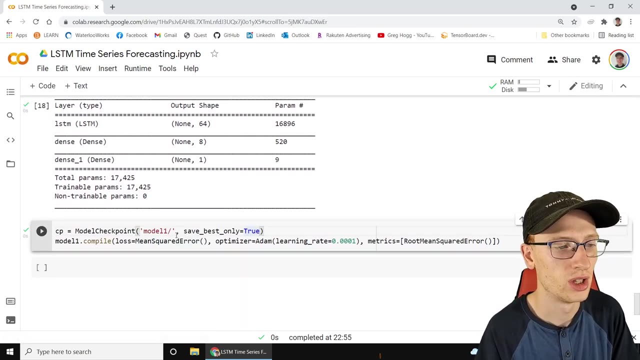 Otherwise it's not going to find its maximum or the local minimums, basically. So we're also going to specify metrics. is equal to the root mean, squared error, bracket, bracket as we defined earlier, And that should be just fine. So here it's going to save only the best model to the model one directory. 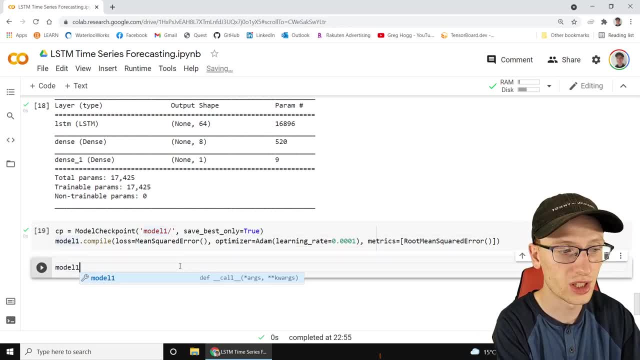 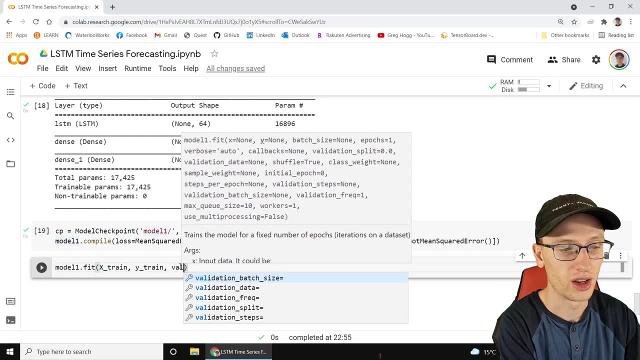 We can load that up pretty easily afterwards. We're going to fit the model model one dot fit with. We're going to pass it X train And Y train And the validation data- validation data- is going to be the X bow and the Y bow. 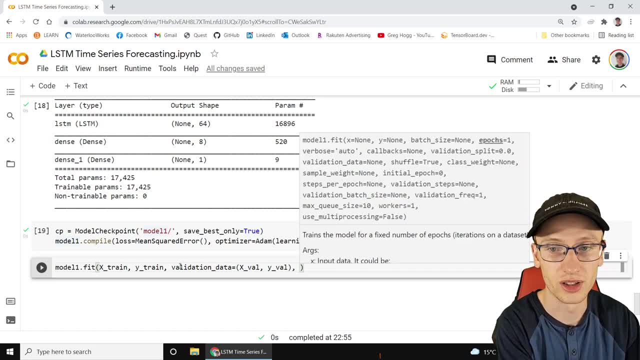 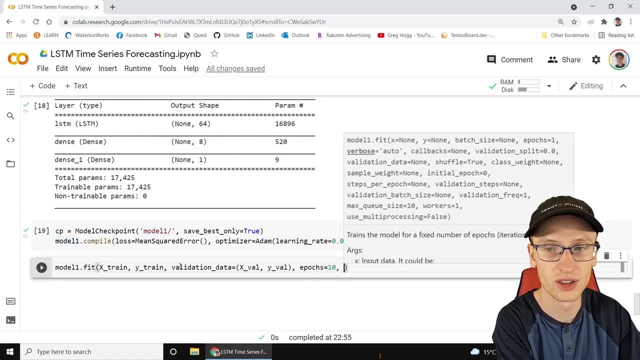 Okay, So it's going to measure the performance on this data set as well, And every epoch epoch is just a run through the dating data set. We'll set epochs equal to 10 to 10 runs through the data set with the training data set. 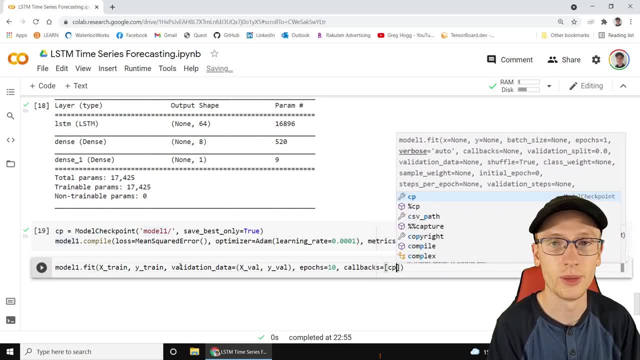 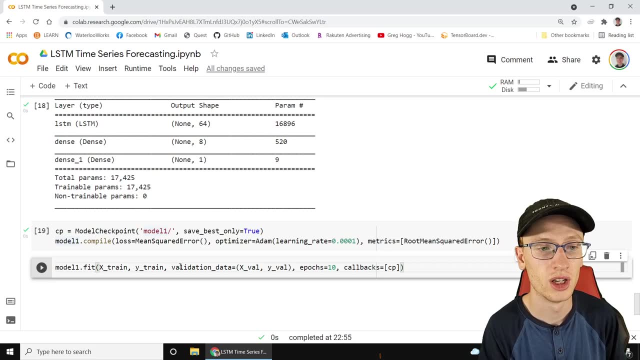 And we want to run this callbacks, just this function. We're going to make sure it calls back this, the CP thing, after every epoch to see if it Wants to save the model. depending on if the model, if the validation loss was higher or lower than it was before, it's only going to save it based off of the absolute minimum that it's seen validation loss. 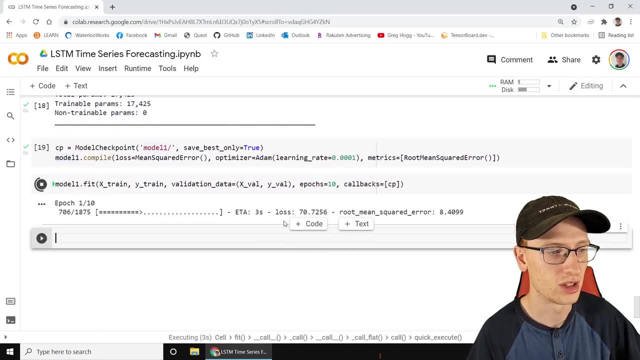 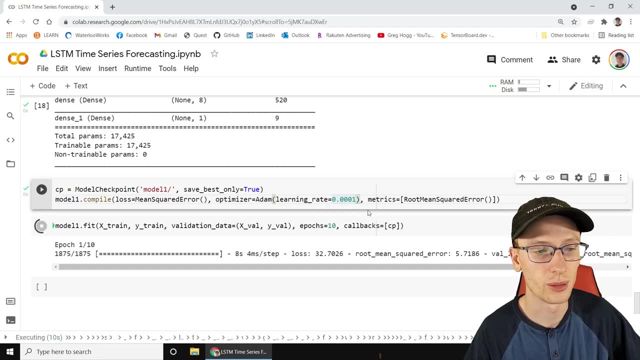 So we'll run that and let's let it watch, or let's let's watch it go. So it's it's rapidly decreasing the loss. It would be decreasing it a lot faster if we were at a bigger number here. but I play with. I played around with this a little bit earlier and I was pretty happy with this learning rate. 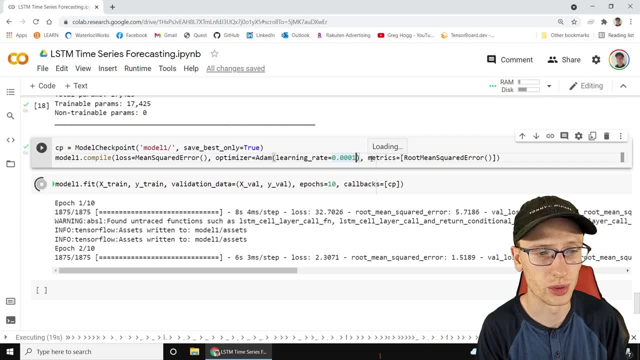 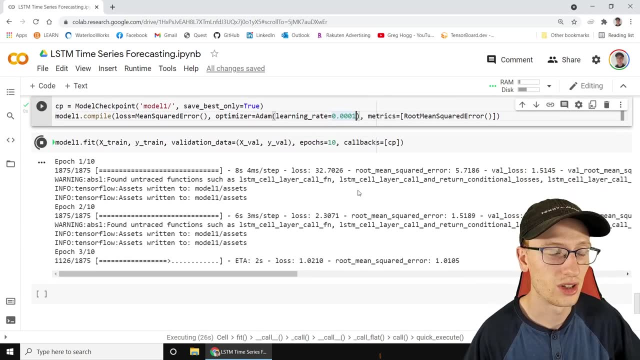 Again as an experiment. for sure, if you want to go and play around with that value and see what you can get out of it as well, then by all means do that. I'm going to let this go for a little bit and I'm just going to cut to after this is done. training and we'll talk about it there. 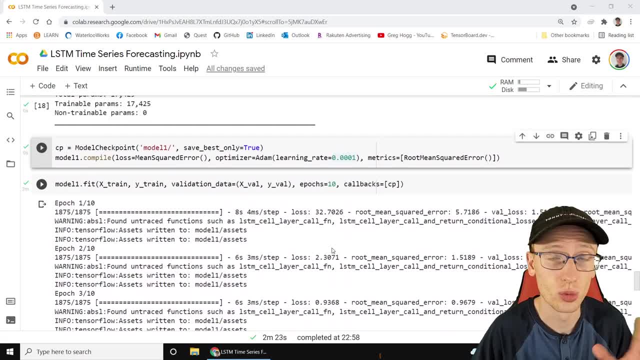 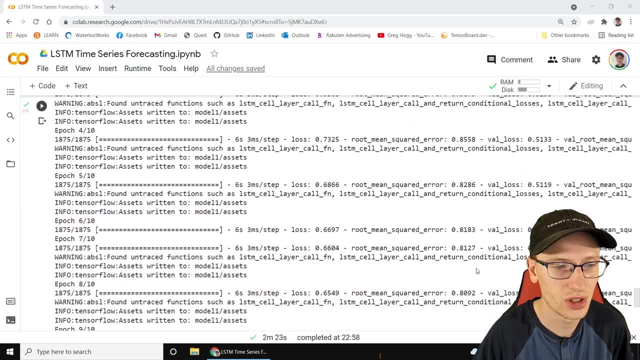 Okay And it appears that we're done training here. I apologize for the absolute word vomit here, but basically, if you find it, we can see that loss went down every single time on the training set, which is pretty common, And sorry for the headache root mean squared error accordingly would go down as well. 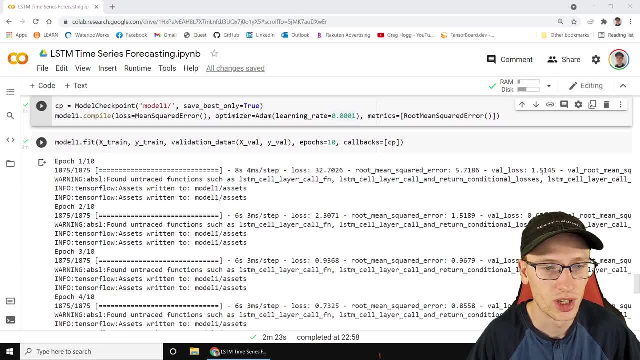 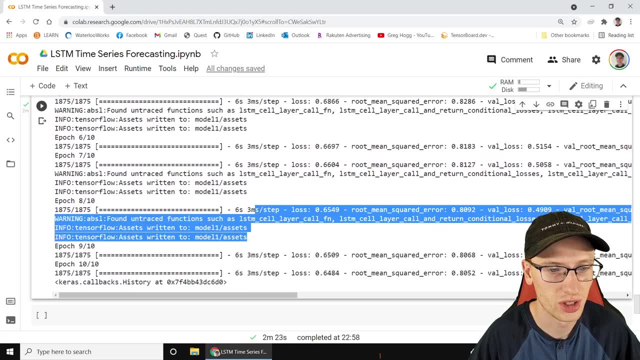 It's just The square root and the validation loss, which is most important, is going down, It's going down, it's going down And it actually, you know it's saved on not quite the last one, but the lowest one was here: 0.4, 9 0 9, and it's saved there. 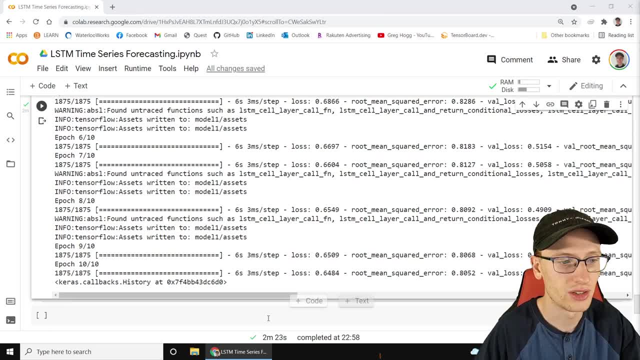 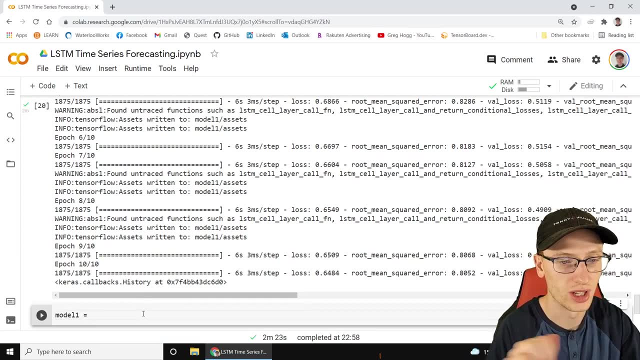 So we can go ahead and load the model that it actually saves. I mean, technically it still has this model in in memory with model one, but we want to load back the one that had the lowest validation loss, And we do that with model model one. 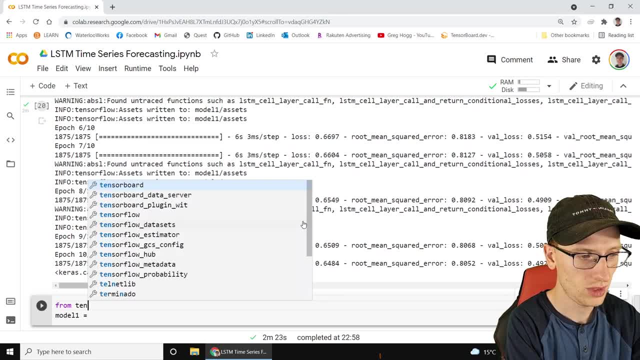 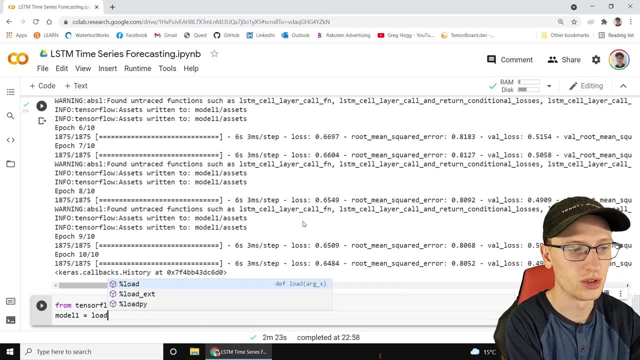 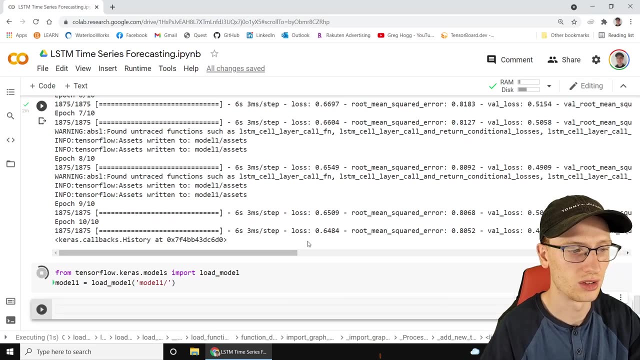 Actually we need a quick import here. We can do from tensorflowcurasmodels. import load model brings the model into memory. Model one is equal to load model with model one slash. give it that directory and it imports it. well, not imports. 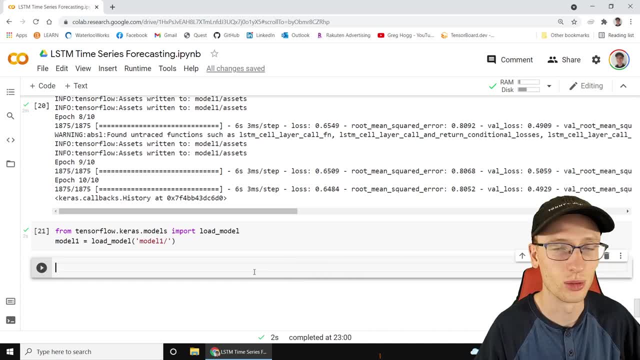 It's someone- someone I know actually uses that term a lot for what this is called. but no, it loads it into memory and there it is. So now what we're going to do is get, just make a pandas data frame, and we're going to make three: one for train test. 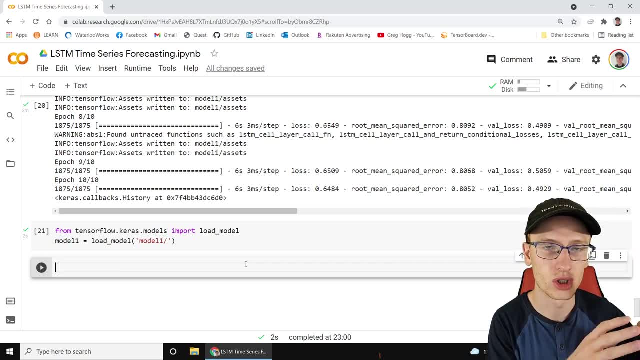 Okay, And validation um for just showing where all the trains, where all the predictions are compared to the actual label. And to do that it's very easy, We can get the train predictions- is equal to model one: dot predict on X train. 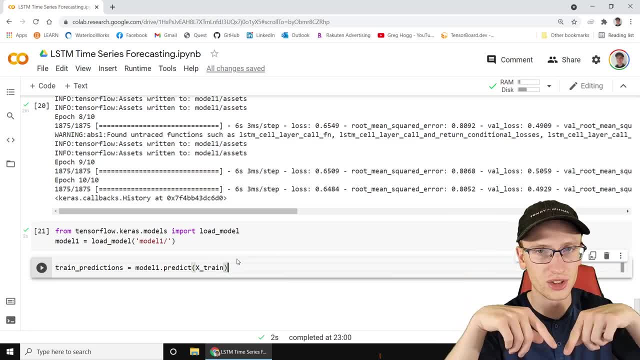 That actually creates kind of that weird thing where we have a vector of of predictions, except each of the values actually wrapped in a list themselves, Like kind of like our input matrix was before. we don't really want that, So what we do is flatten and that just makes- uh, it gets. 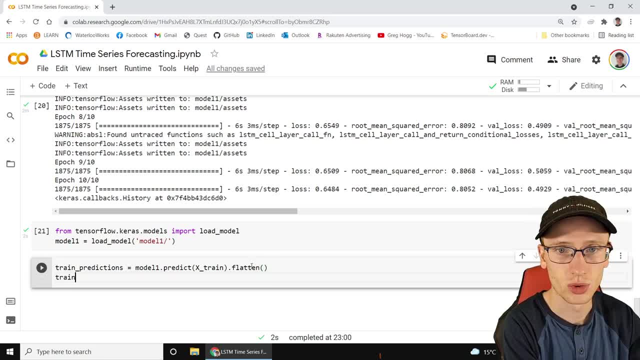 Over to those inner brackets like that, And we will also get train results, which is going to be our pandas. data frame, train results- is PD, dot, data frame, Uh, data frame, uh. data is equal to. we'll make two columns here, just train predictions and the actuals. 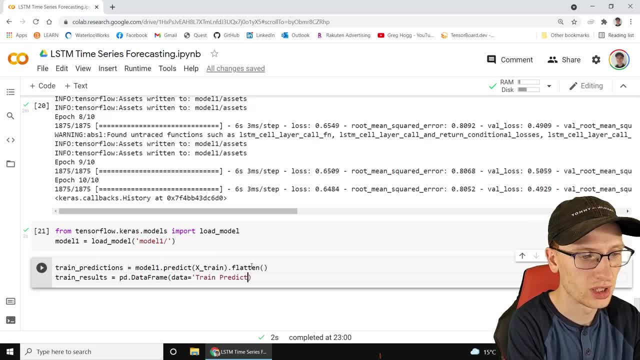 So this is going to be called uh, train predictions and that value- uh, sorry, I missed the. the brace for the dictionary data- is going to be this Dictionary, Where- here's the first, here's the first column, train predictions is going to be just, um, well, train predictions. 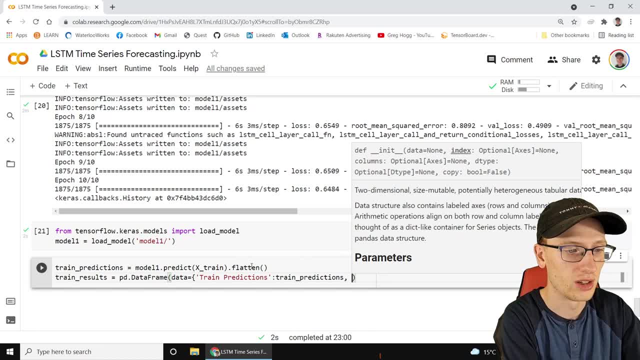 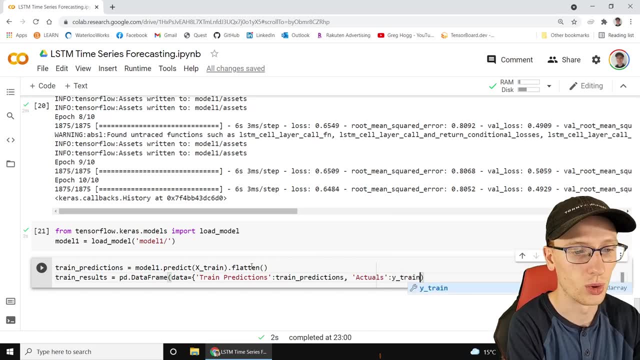 That's not really that surprising. And the next key uh value, which is the next column, is going to be actuals and we will set that equal to. this is just going to be why train is the actual labels And we can output this with train results is invalid syntax. 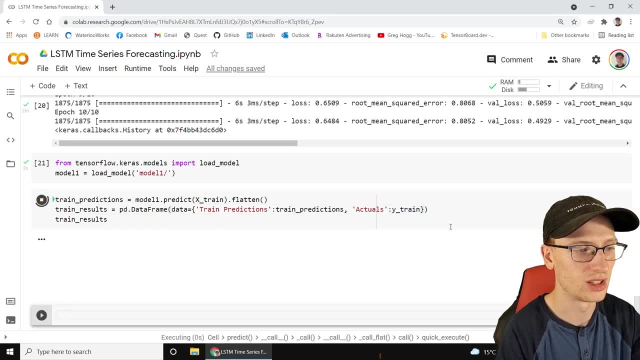 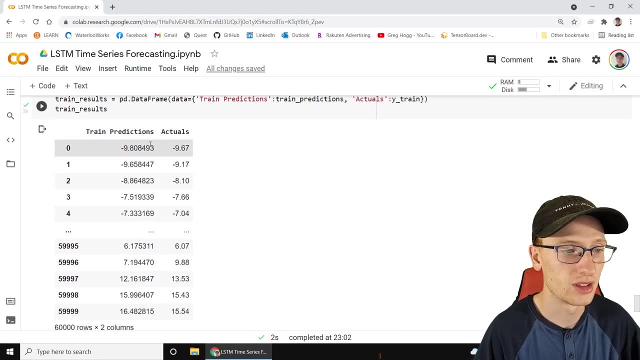 I always do that. That is a brace and then brackets, and that should be right. Okay, it takes a little bit of time to make the predictions not too long, and here you go. we have a data frame that has compared to the predictions to the actuals and, unsurprisingly, as we saw on the loss, since the loss was pretty good, uh, it's pretty low. you know, we're pretty accurate here. 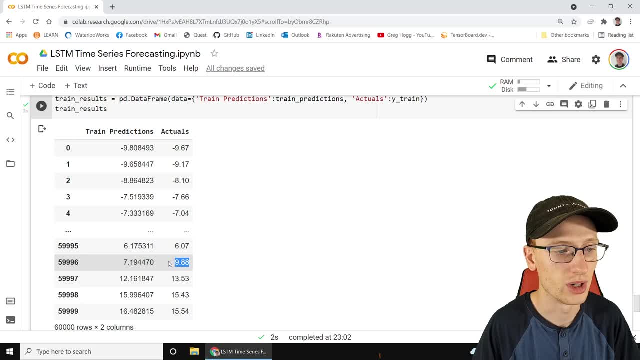 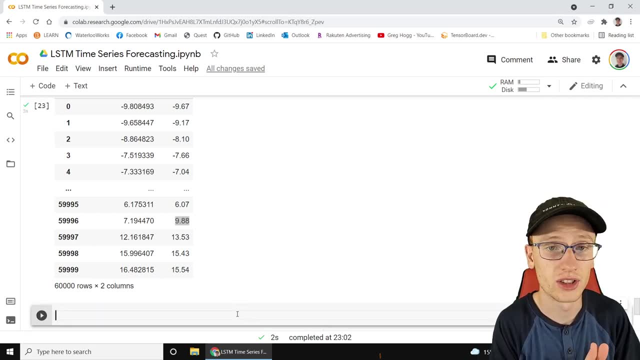 There's some, some bigger mistakes, like 7.1, uh compared to 9.8. Uh, but in general, you know it's pretty darn close and let's actually take a little bit about uh. look at the plots a little bit. 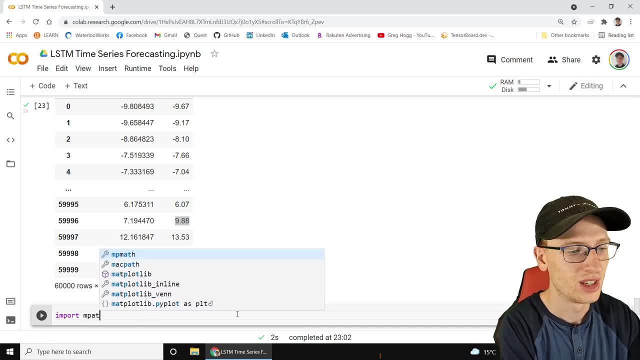 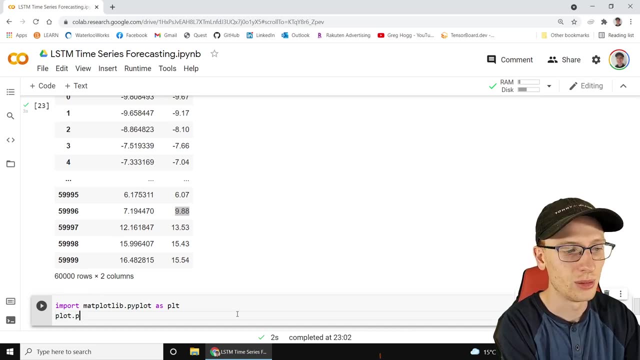 So plotting, you know something very easy. not my favorite um plotting Library, if you guys know me well, but import math, what lived up high plot is PLT Cause, it's nice and easy. PLT dot, that's plot, dot plot. PLT dot plot. 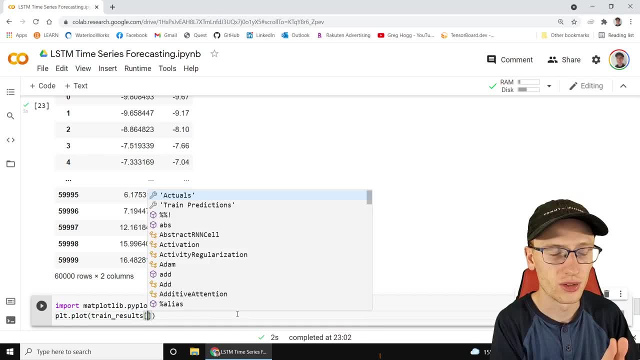 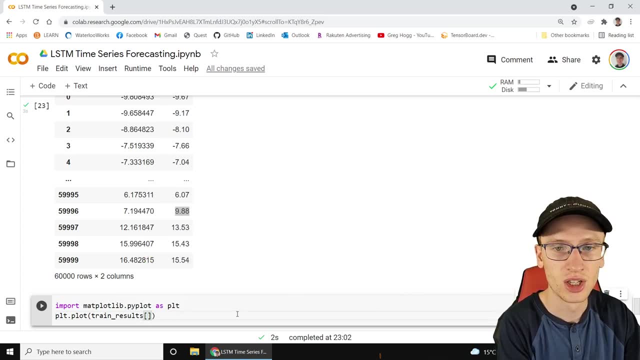 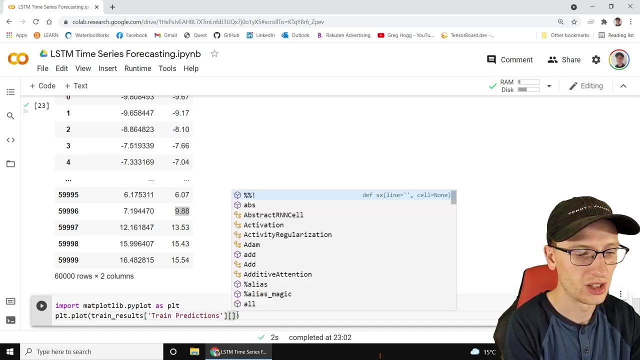 We will plot the train results. So we're just plotting a curve that shows both the, the, the actual predictions compared to the uh or the predictions compared to the actual results. train results- sub train predictions. plot that column And then let's maybe only take the first a hundred or so, just cause it zooms. 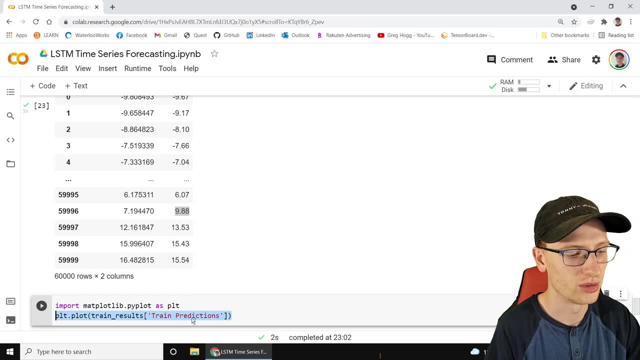 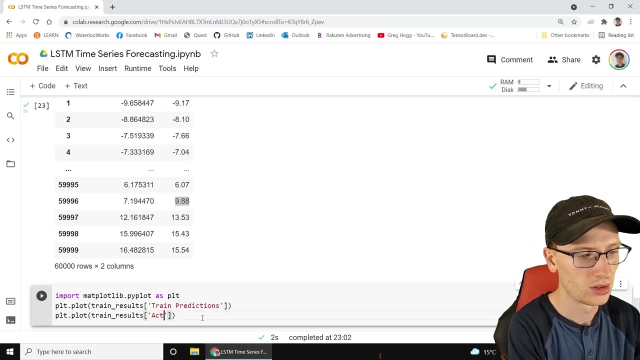 Actually, let me show you. let me show you what it looks like without that, just to kind of prove to you why we want to change it there. And then we'll do train results sub actuals, Okay, So comparing the predictions to the actuals, you can see it looks like this. 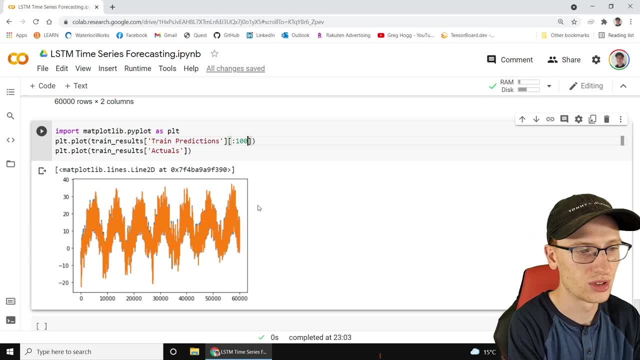 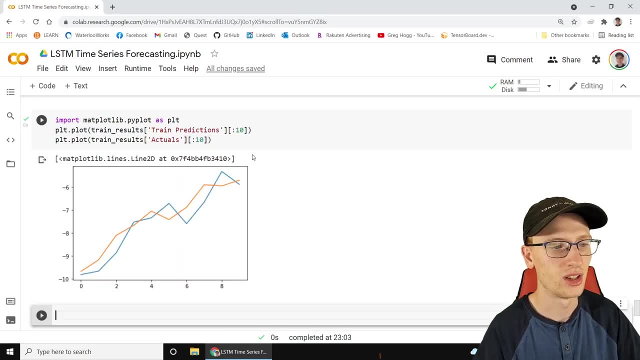 So that's why I kind of want to show maybe just like a hundred results or maybe honestly even just 10 random ones. So this is that's not really random. That's the first 10.. Uh, but looking at the first 10, we can see, you know, it's pretty close. 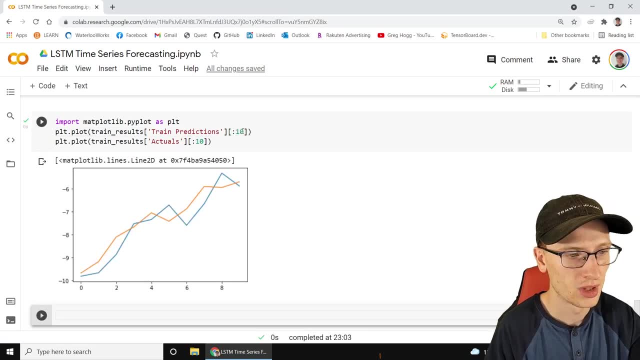 And now if we zoom out, uh, you know a little bit more. That's not what I meant. Uh, if we look at, you know maybe the first a hundred results, you know we can see we're still pretty close. 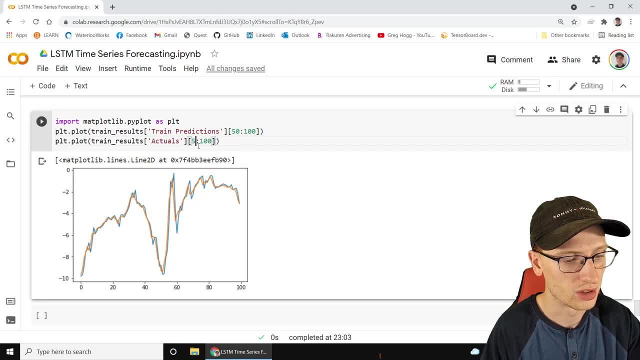 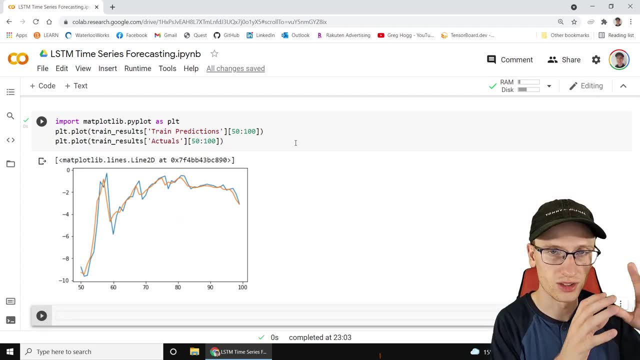 And if we were to look at, say, you know 50 to a hundred the the second 50 is, you know it follows it very well. So it's training. it's trained off of the last uh. you know five hours of uh of data and it's able to predict, given five, the next one very, very well. 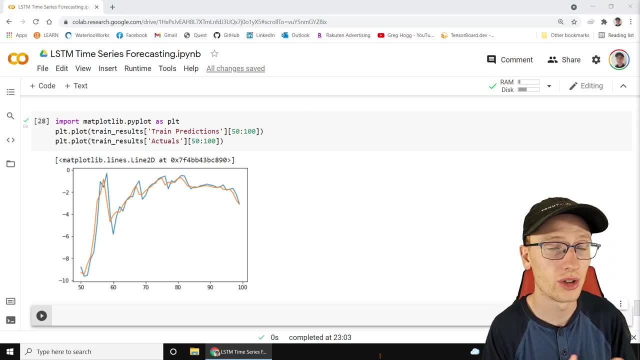 Okay, So that's quite interesting, And now we are going to look at how it did on the validation data. So that's training. Uh, we don't really care about how well it did on training, because it's already seen that data before. we want it to generalize. 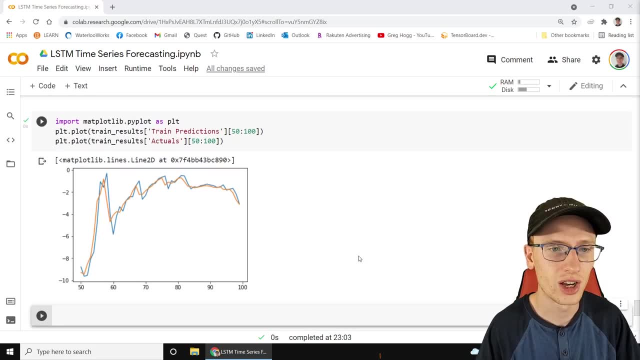 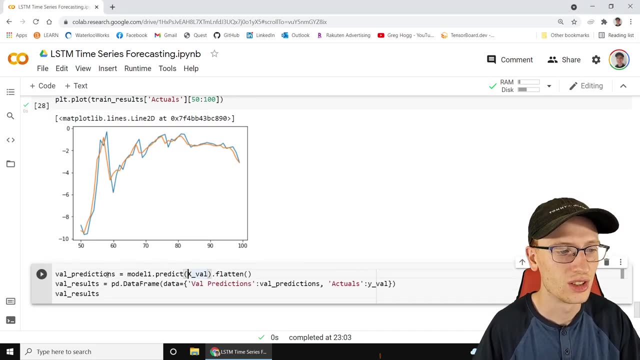 And so to do this, we are going to copy um. actually, to save time, I'm really just going to copy the stuff that's from my other notebook here. It's really common sense, because we're just changing tests or train, changing train to Val every time. 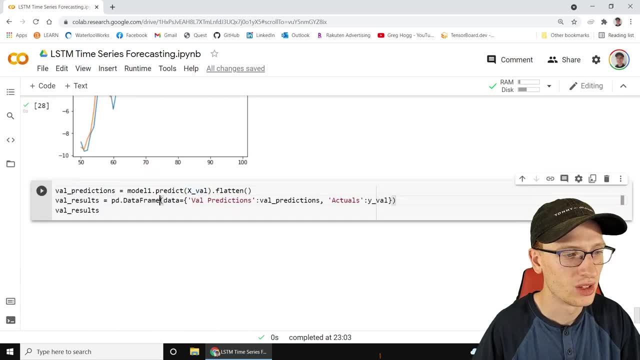 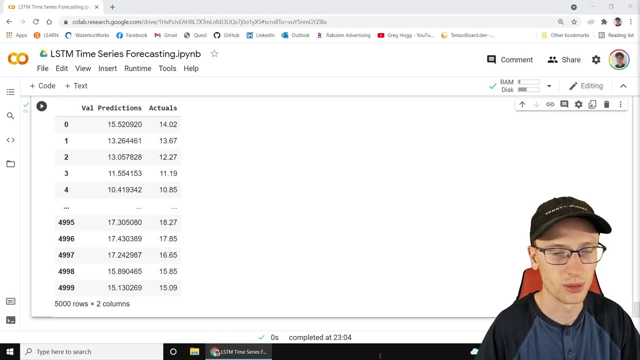 So every time we see train, train, train, we're just changing it to Val. So here we can do it like that And there you go. So that's, that's the comparison. We can get the plot as well. I'll just look at the, say, the first a hundred validation results like that: 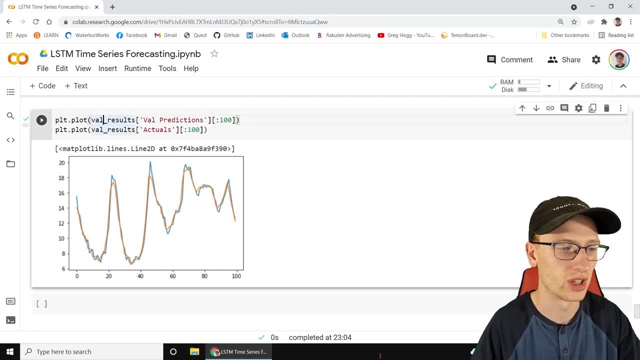 And again, I'm just changing the above code to Val. It's really nothing crazy. You can look at it if you want to, but uh, you know we're very, very, very close. It's awesome. And then, finally, what uh has really, really never been seen in the slightest uh is the testing test data.